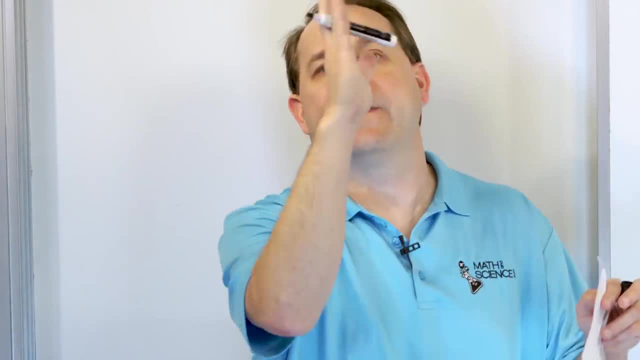 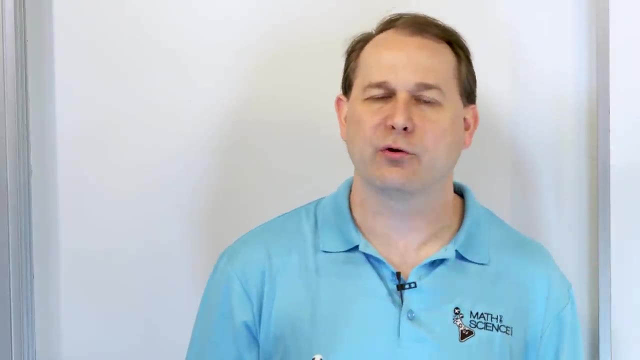 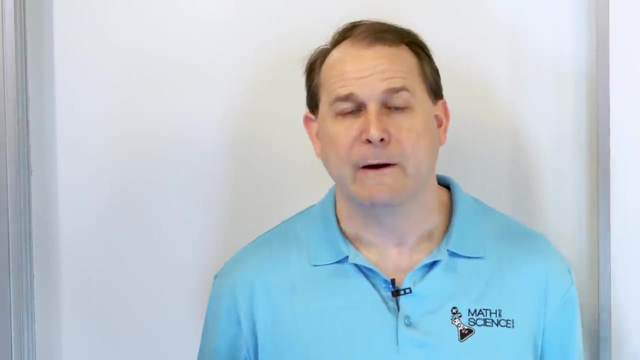 what it is is, if you take a circle and you chop, going around, that circle into 360 equal pieces, then one of those little pie wedges of a circle after you chop it up like that is what we call a degree. Now, why is it 360 degrees? Why isn't it 380 degrees? Or why is it, you know, not 270? 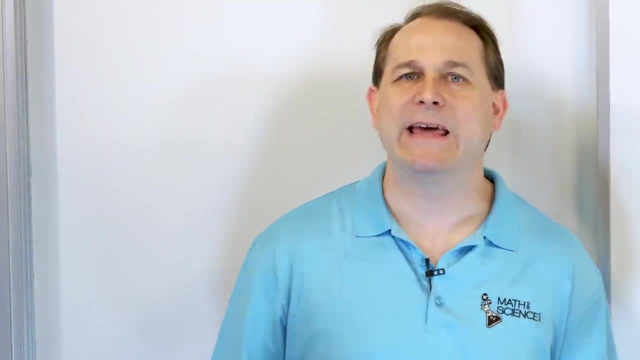 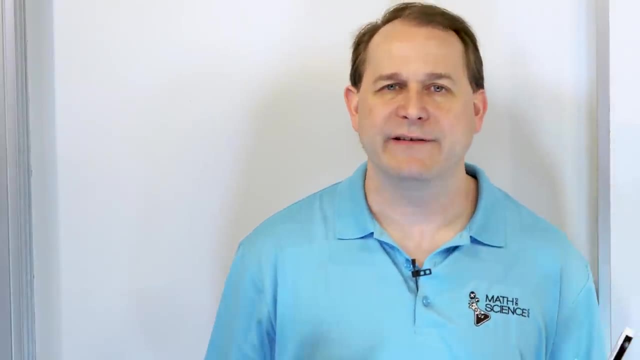 degrees. Well, that goes into the history of math and map making and other things And why that is the case. we're not going to talk about the why. we're going to talk about what it is. But ultimately, the 360 degrees is just the measure that we have landed on here. It doesn't make a 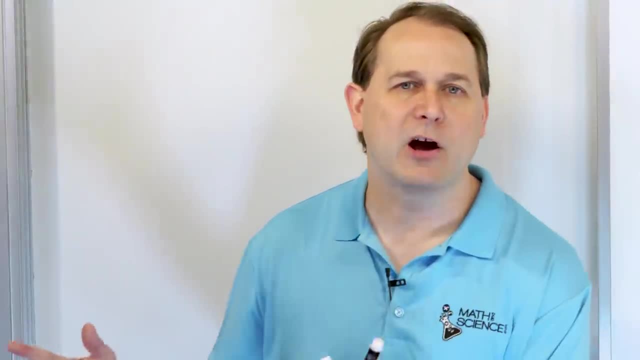 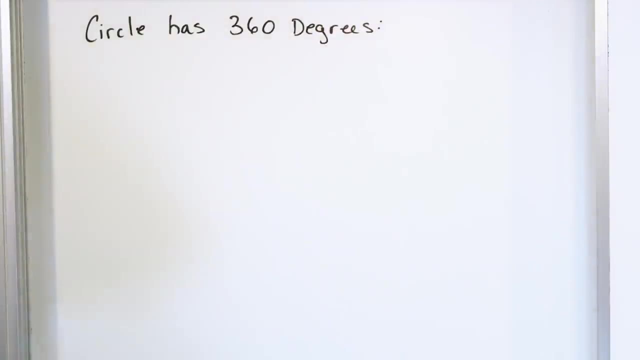 lot of intuitive sense why it's 360 degrees. Later on we talk about radians that will make a lot is defined the way that it is, But for now we're only talking about degrees, And so we're just going to take it as a fact that the people that you know figured out geometry and map making and 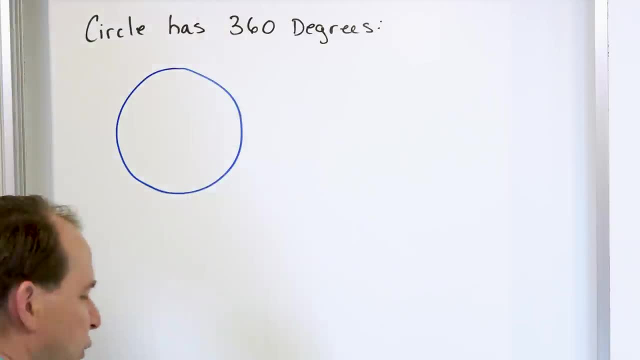 surveying and things like that, in the past settled on 360 degrees For a very good historical reason. we're not going to talk about the historical reason here, But what it basically means is if I, if I have a circle like this, if I start at one point in the circle like this and if I traveled. 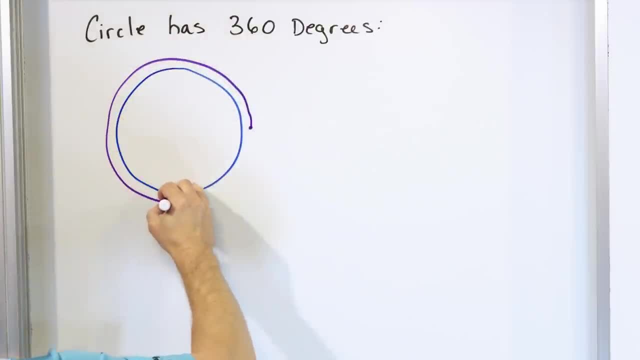 all the way around, like this, all the way around back to the circle. I'm going to have a circle to my starting position, So my arrowhead is right here, And what I mean by that is if I kind of take from the radius here of the circle and start at this location and sweep out all the way like a. 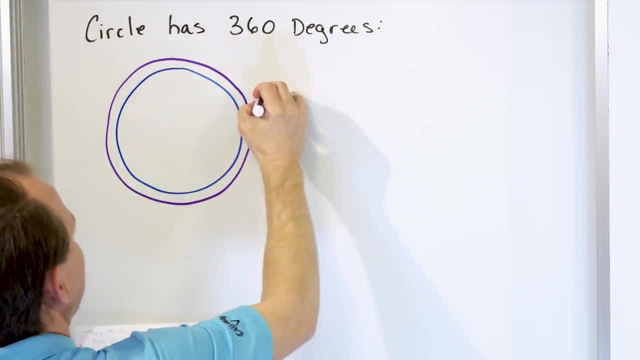 clock all the way back to where I started with. this is what we call 360 full divisions of that going around the circle. we call that a degree And obviously we can talk about radian measure which splits the circle into it's going to end up being two pi radians. you see, pi is involved. 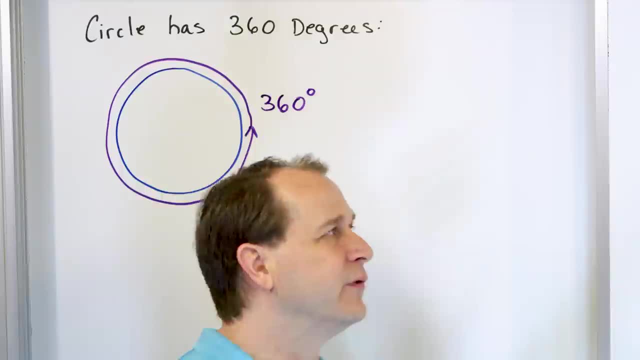 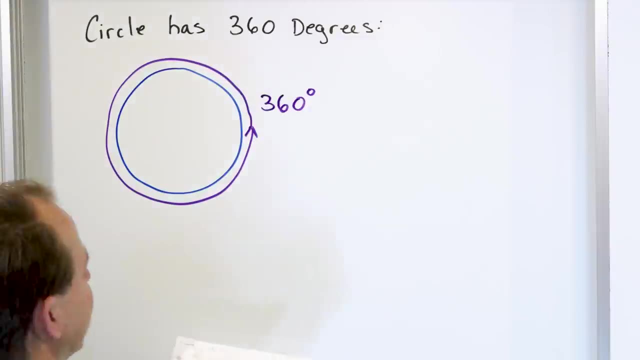 when we have radians, But we're going to save radians for later because I want to get the through the fundamental concepts first. Right? So this is a full circle, right, But angles in general, like in triangles, are not a full circle. So what we have here for in general is, if we have 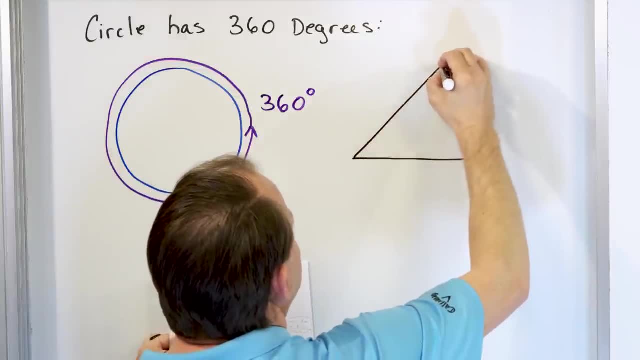 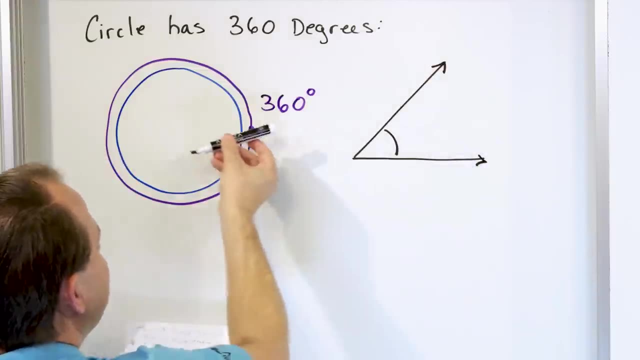 an acute angle or something, then we might have an angle that goes up like this: it's not a complete circle, because this angle measure that we're going to ultimately be talking about is only a portion of a circle. you see, the entire circle goes all the way around to 360 degrees, And then 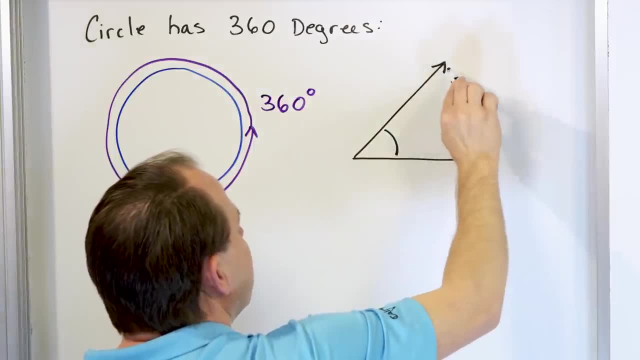 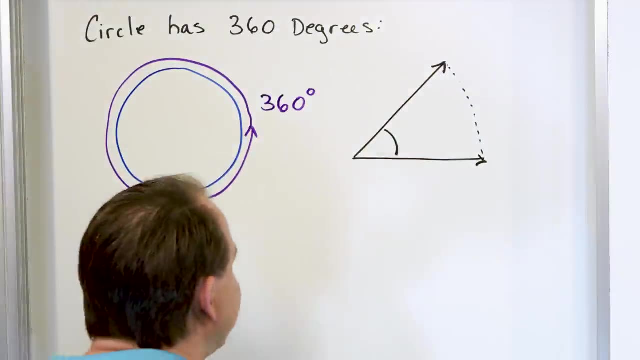 this amount, that this thing is open. if you can imagine like a circle kind of going like the boundary of the circle kind of going like this, this is just a fraction of going all the way around the circle, So it's not 360 full degrees In this particular 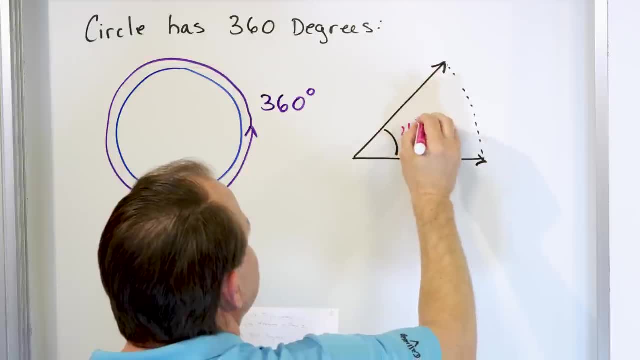 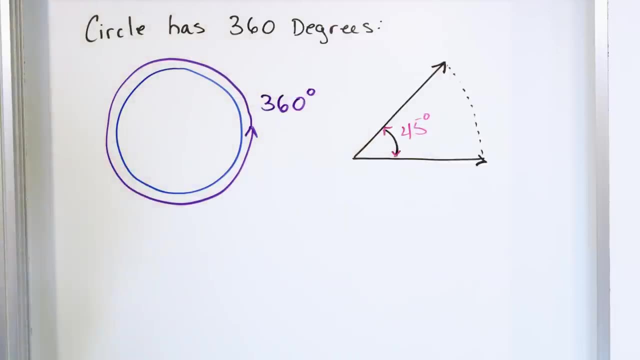 case it might be something like 45 degrees, let's say, and the angle measure is measured from. you know this line up to this line, right? So you need to kind of start getting used to measuring these angles, opening and closing in the following way: we have two sides. 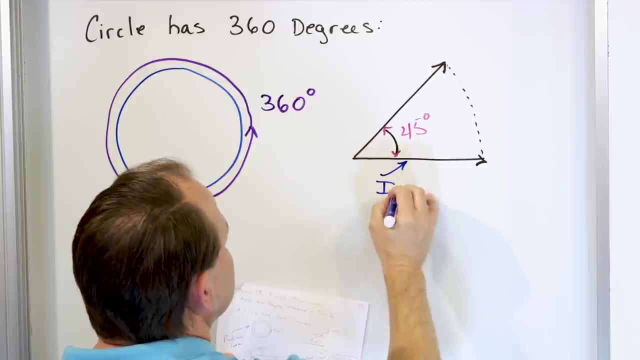 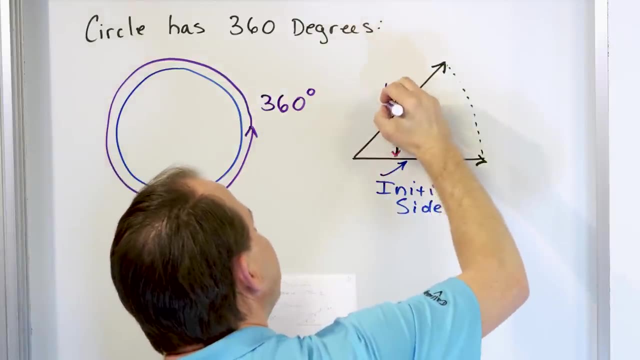 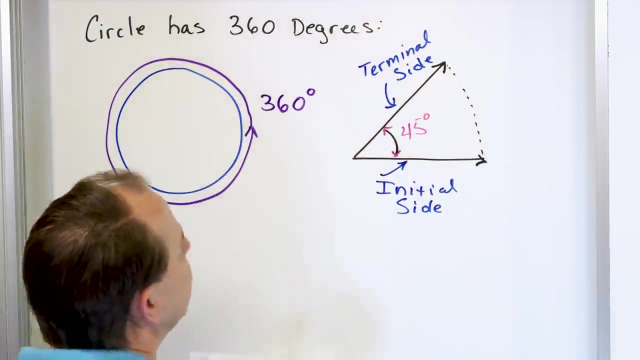 of this angle, this side right here is called the initial side, And then over here, when we get up to where we're kind of going, this part is called the terminal side, initial and terminal. Now, in this part of math when we kind of get out of basic geometry, 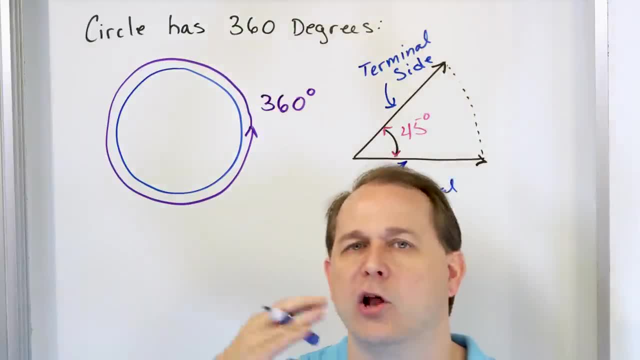 and we're starting to talk about really weird angle measures that go all the way around the circle. we generally have to start measuring the angle from something like this: So we're going to be measuring angles from some known location. So, from here on out, we're going to be measuring. 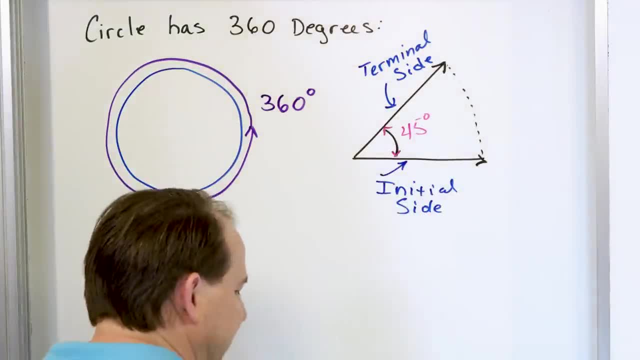 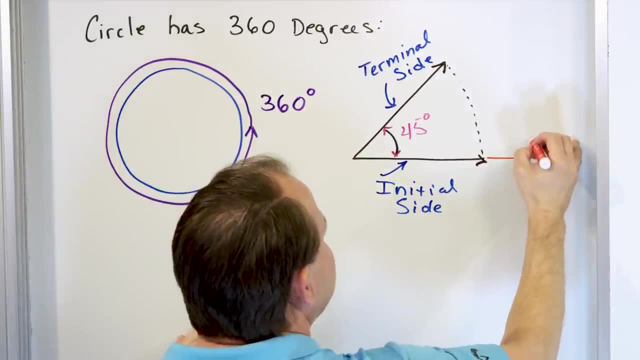 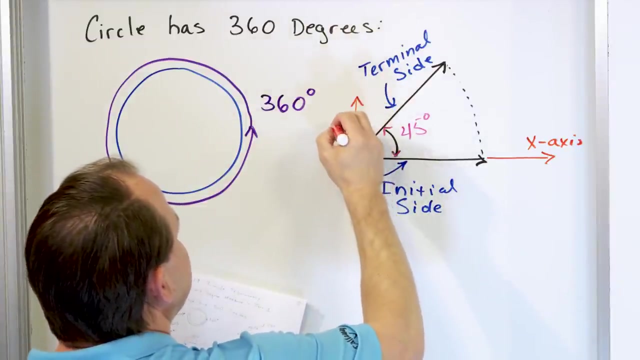 angles from the positive x axis. we have to have a starting point, So we measure it from the positive x axis. What I mean by that is this: imagine that this is an x- y plane and the x axis actually continues on here. So this is the x axis right, And so you can imagine this part right here, this. 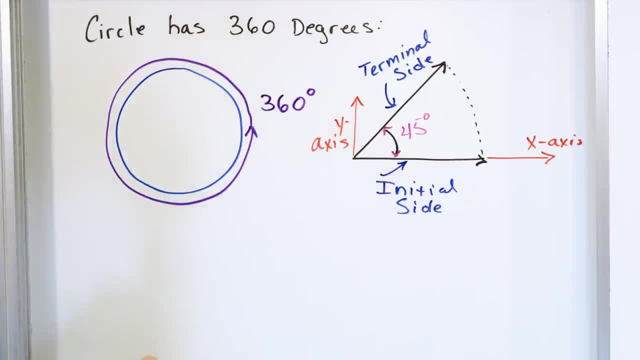 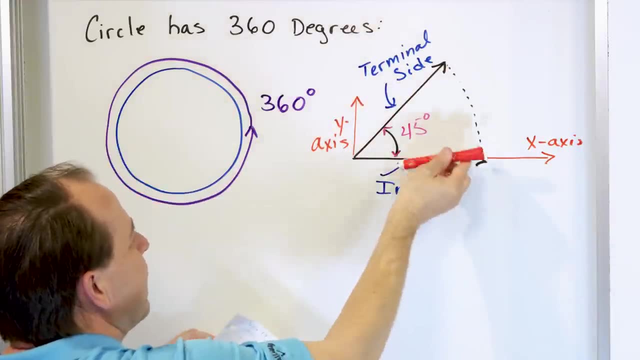 would be the y axis, something like this. So this, going from the x axis to the y axis, this is 90 degrees, And about halfway through there we stopped- roughly halfway- I'm not exact in my drawing here- right halfway. So this is half of 90, which makes this about 45 degrees. 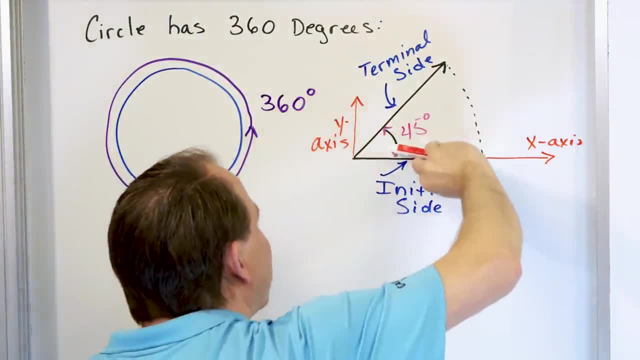 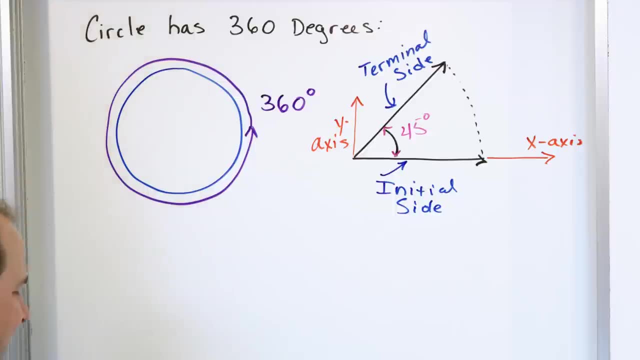 And then, of course, you can continue past 90. And kind of go all the way around, in which case you get back to 360 degrees. So these are little angles that we've used and looked at in the past, for instance in triangles, But here, when we get into the trigonometry and 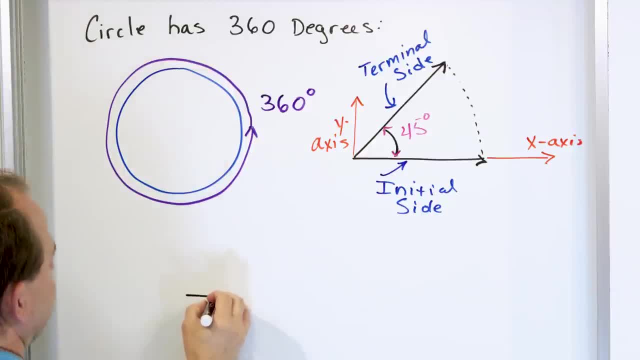 kind of more advanced learning. we have even larger angles that we deal with, And that's what we're going to talk about in a little bit. So let's take a look at an example here. So here we have this initial side. Instead of opening up and stopping somewhere here, let's continue on. 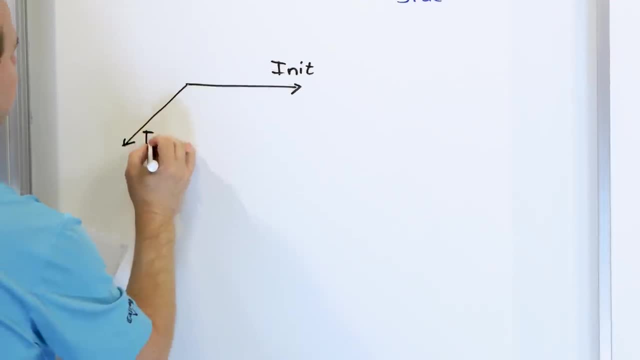 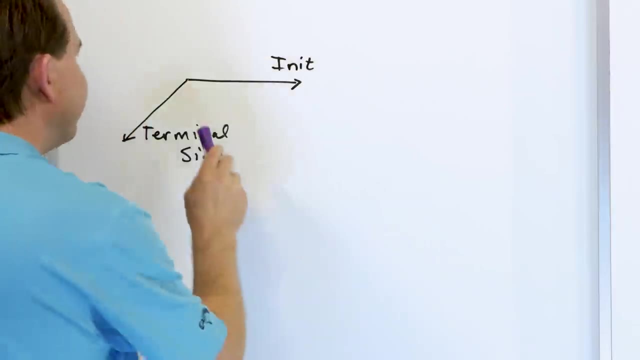 and measure that angle all the way down. Let's just talk about an example coming down here. So let's call this the terminal side. Now you might be tempted to talk about the angle measure in here, And you of course, can take a look at that angle right here. But in general, you want to? 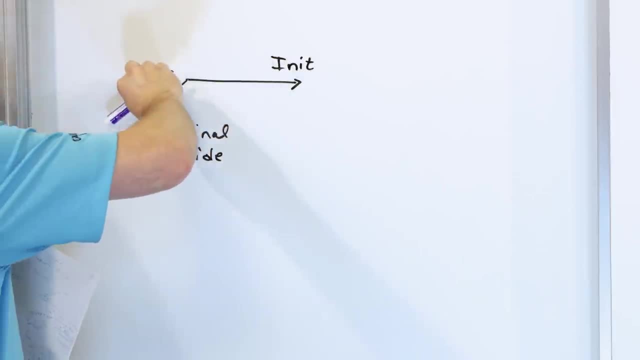 go in a counterclockwise direction. Remember, clocks go like this right, So counterclockwise goes the other way. So we want to take a look at the angle measure that goes through this. So if over here is 90 degrees, then over here would be 180 degrees. That makes sense. 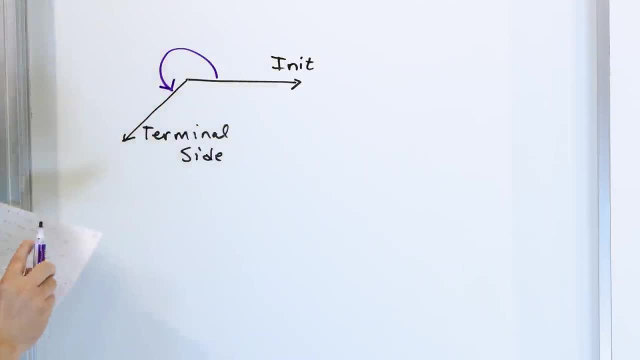 180 degrees over here And this is just a little bit bigger than 180 degrees. So in this example, this is 225 degrees, So it is perfectly valid to have an angle larger than 90 degrees, an angle larger than 180 degrees. Now it's a little weird. the first time you see that. 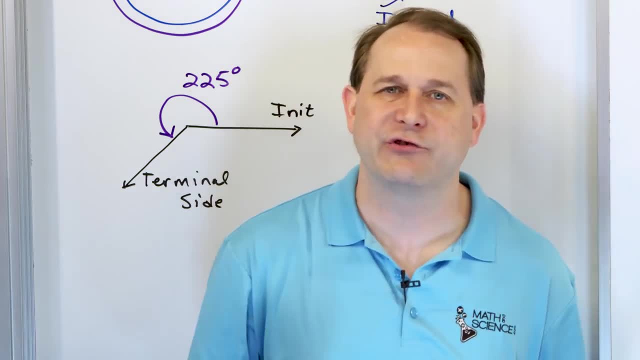 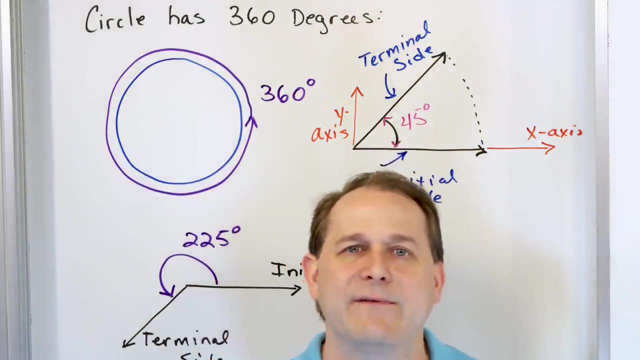 because usually in geometry you're only talking about little angles inside of a triangle And they're always these or often these little acute angles. But in trigonometry and precalculus and calculus we have angles that go way beyond 90 degrees, way beyond 180 degrees, all the time. 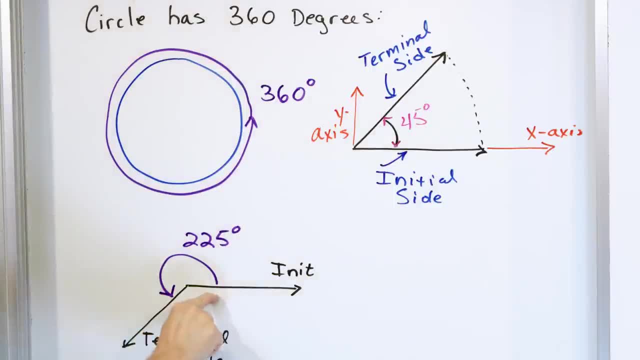 So it is true that you do have a smaller angle in here, and we could define that. By the way, it would be 360 degrees minus 225.. That would be what this angle is, because going around is 360.. So if we subtract that away, that would be that angle. Of course, we could take a 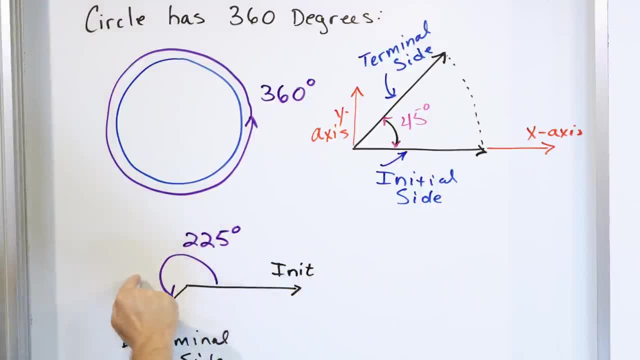 look at that. But in general, we're measuring counterclockwise from the initial to the terminal side, And they could be large numbers like this, which leads me to the next thing that I want to write down. that's important. So when you're measuring angles, when you have something like 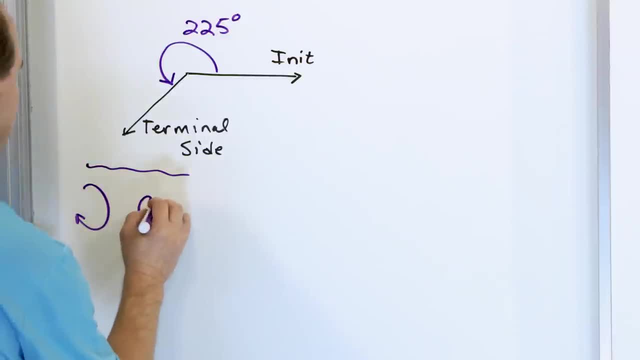 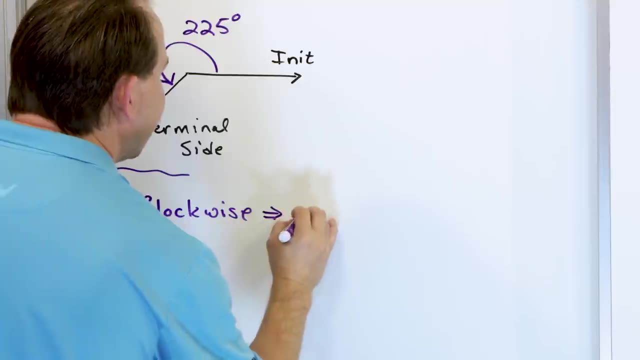 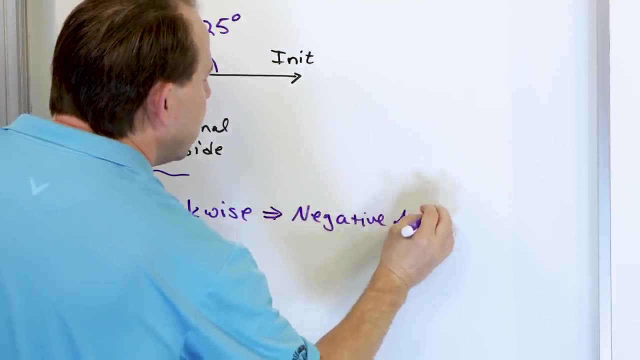 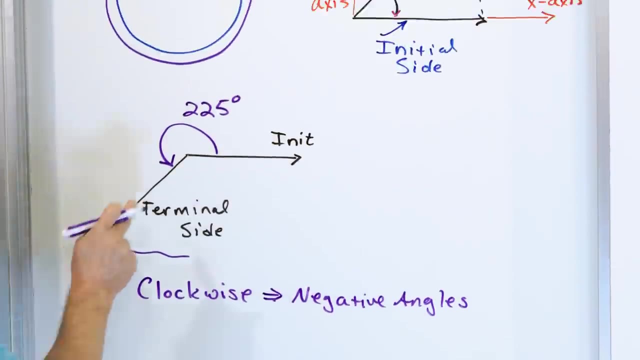 that away, that would be that angle. So if we subtract that away, that would be that angle. Angles: That's the other weird thing. When you get out of geometry and you start getting into trig and precalculus like this, you can have negative angles and positive angles. Now, in all of these, 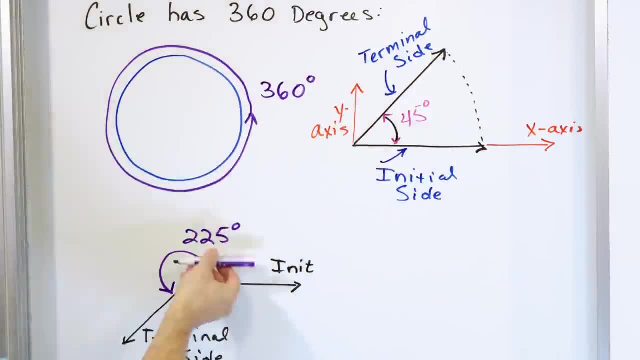 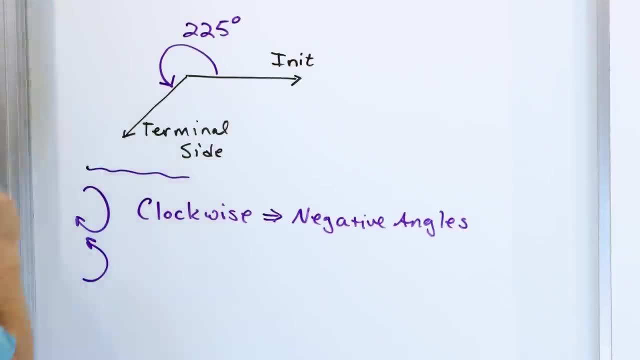 examples: we start up here and we're going counterclockwise, counterclockwise, counterclockwise. So the other direction, like this, is counterclockwise. This is the direction we've been measuring for these guys right here. So counter, I'm going to put a C clockwise, Okay. So 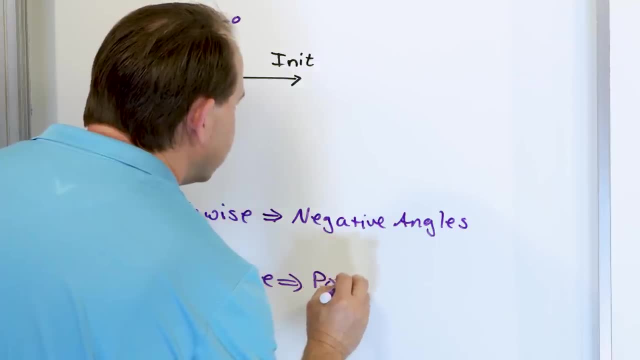 So the other direction, like this, is counterclockwise Okay, So we're going to put a W, counterclockwise Okay, So of these guys are always going to be positive angles. It's extremely important you understand that, you know and the basic ideas. 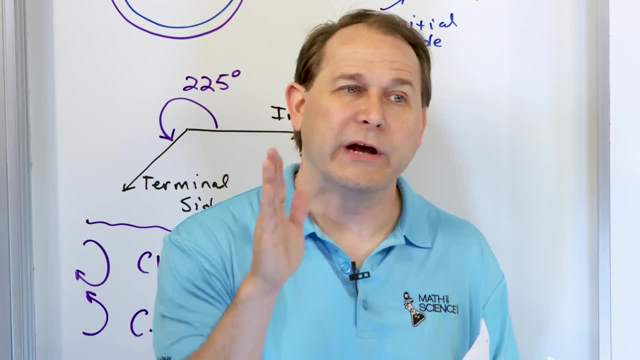 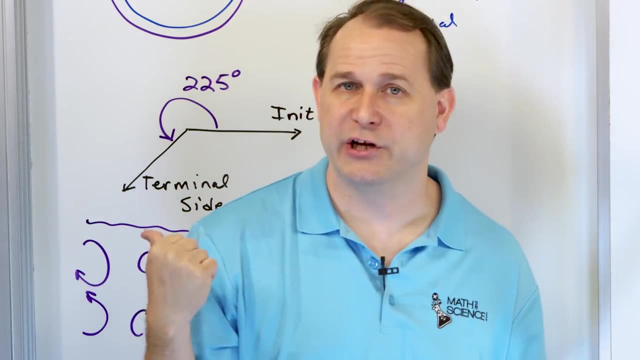 United States of algebra you learn what a positive number was. that's going along to the right, going on the number line towards the right, And negative values those are going the other direction, past zero on the number line. Same thing for y: positive. 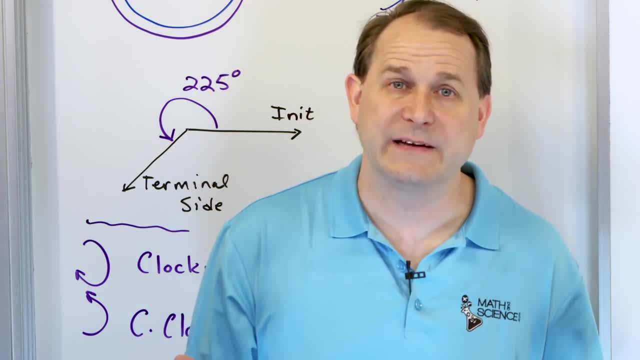 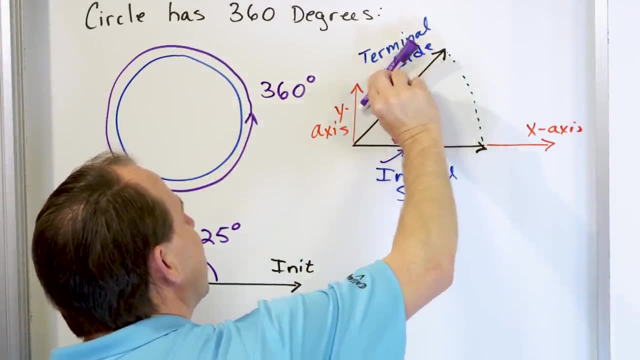 is up, negative is down. You had to learn all that in the beginning. So here we're talking about something similar. It's extremely important for you to understand If I start at something- Magellan Bahier was a- If I start at some initial side and I measure angles in the counterclockwise direction. this 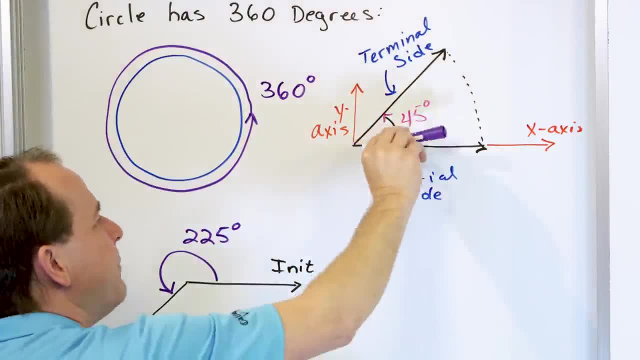 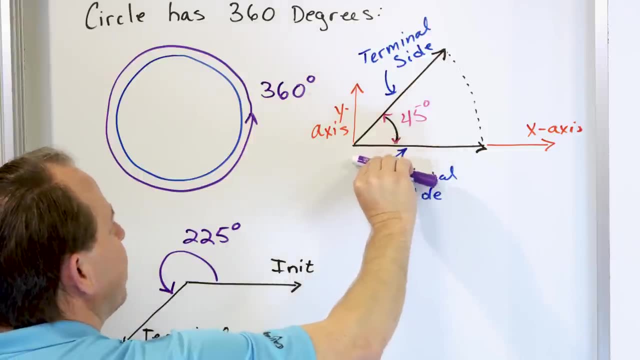 way. I'm measuring by definition, by convention, positive angles. That's why this is positive 45 and positive 225.. But if I start at this initial side and I measure an angle below the axis like this, then I'm going the other direction in the clockwise direction. 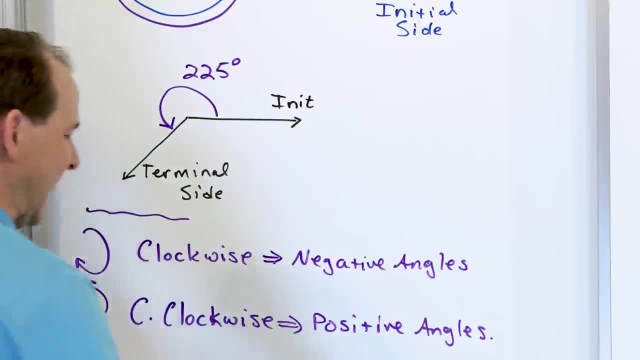 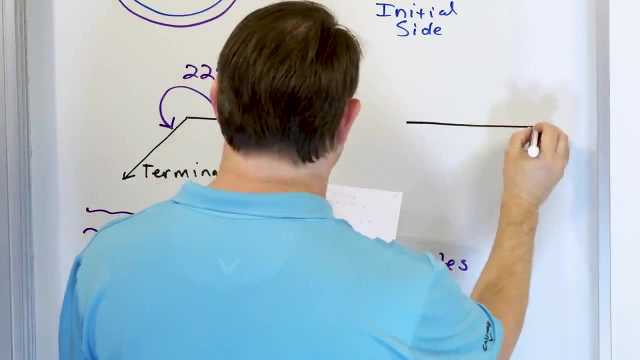 I'm going to, by definition, define and be looking at negative angles. So let me give you an example of that. So if, for instance, you have the initial side right here, so I'm going to call this initial- Remember they're always measured relative to the x-axis, like this. so the initial side, 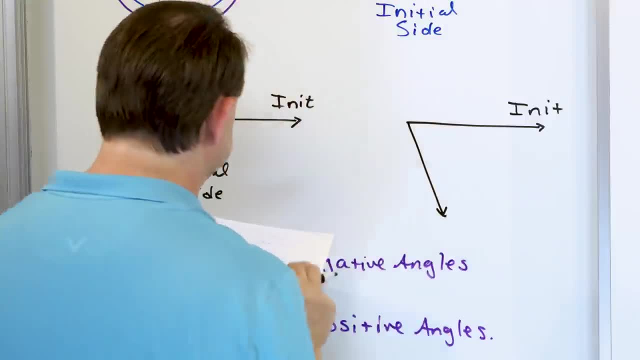 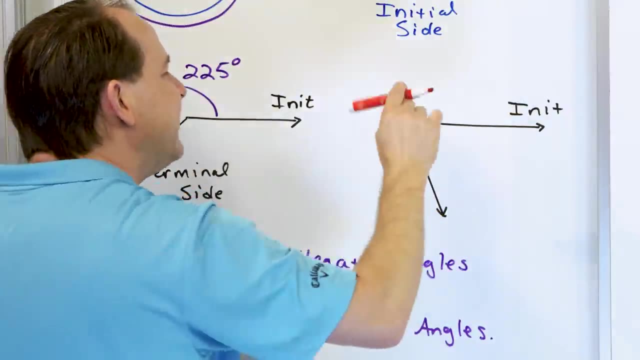 And then I have an angle that comes down something like this, But for whatever reason, I do not take and look at this angle over here. That's a positive angle. Instead, I start here and I go and look at the angle below. 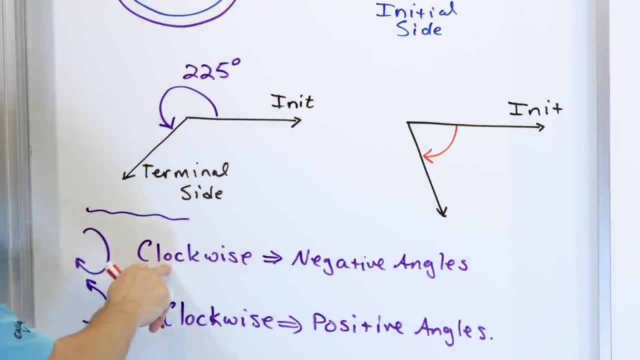 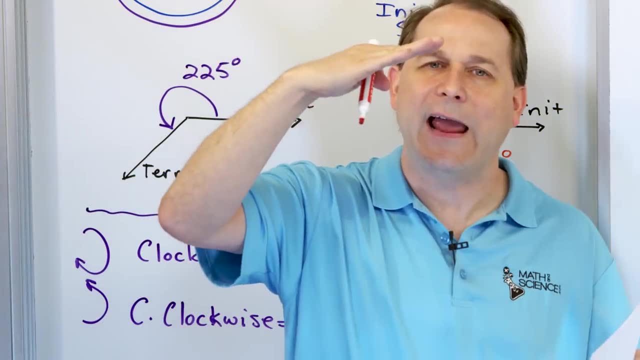 I start sweeping down below like this, in a clockwise fashion. This means this is a negative angle, So it's Negative 60 degrees in this case. So when you see negative angles, it just means angles that are measured below the x-axis. 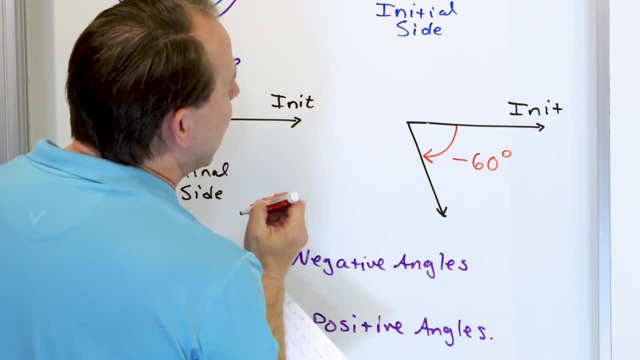 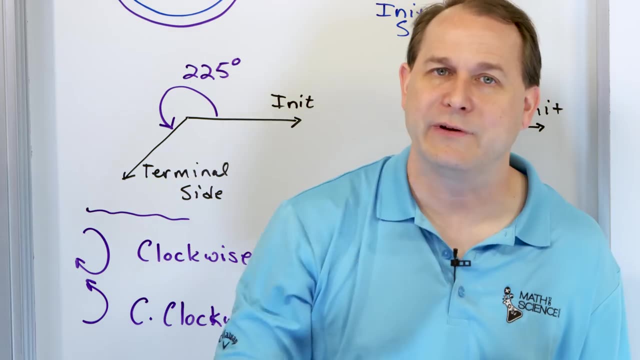 And these angles. of course you can measure negative angles all the way around, Right. But if you start here and you go in the counterclockwise direction, you're measuring positive angles. So one direction, you're measuring positive angles. the other direction, you're measuring negative angles. 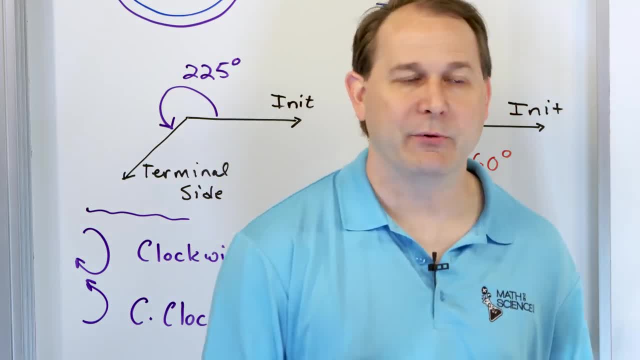 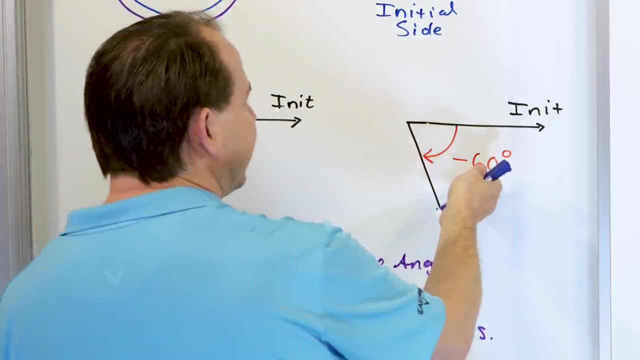 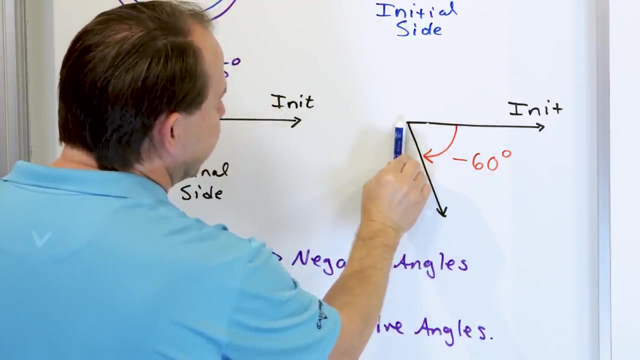 You're never going to get away from this idea in math, So you have to remember that. OK, So let's take a look at what this actual angle is. We just said it's about negative 60 degrees. That makes sense, because if you imagine this vertical line being here, this is about 90 degrees negative 90 degrees. 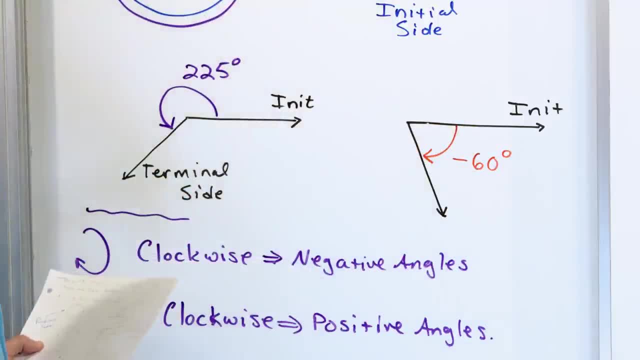 And so it's not quite there, So it's a negative 60 degrees. OK, Now I want to describe something to you, and that is the idea that we are measuring the angle from here to here, And so it's a negative. 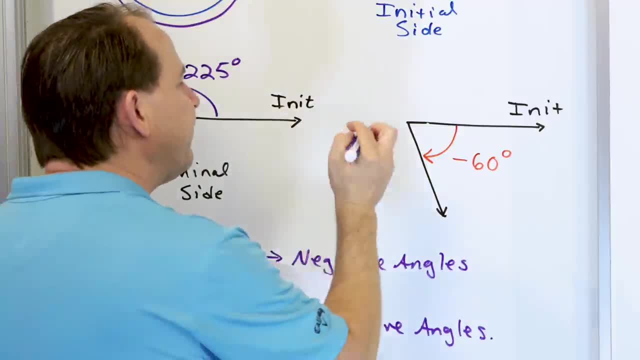 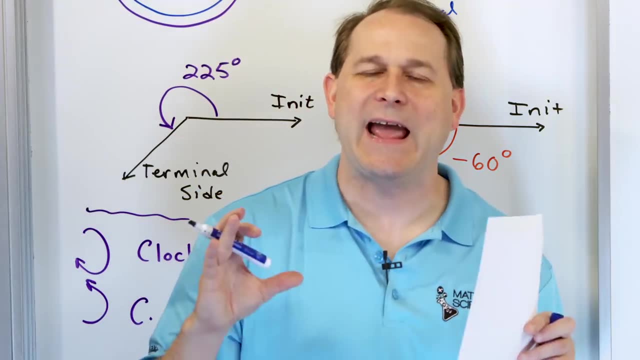 And this is if you get a protractor. it's about negative 60 degrees, But we're perfectly free to measure this angle in the other direction going the other way. It's perfectly fine to define angles measured two different directions. OK, When you measure going below the x-axis, it's negative measurement of angles. 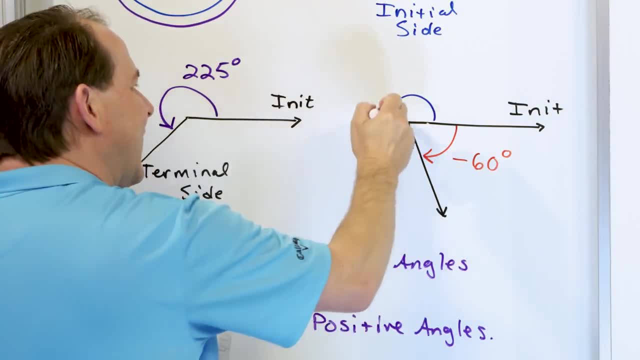 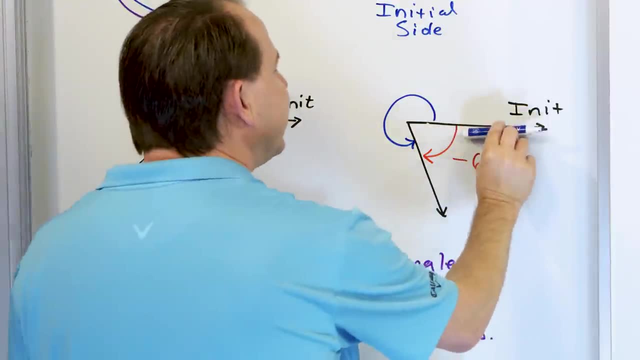 When you measure it going the other way, it's a positive. So how would you figure out what this positive angle is? if I were to start here and measure in the positive direction, OK, How would I do that? Well, you know that this line right here is the zero spot. 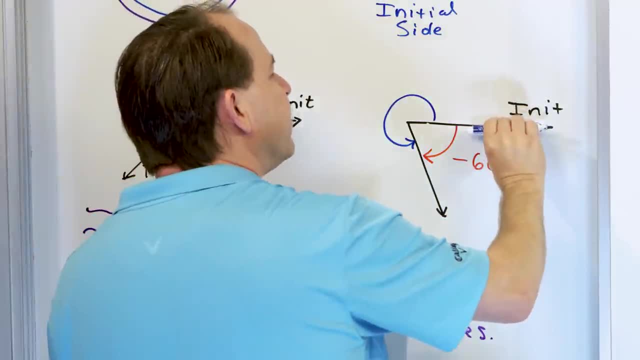 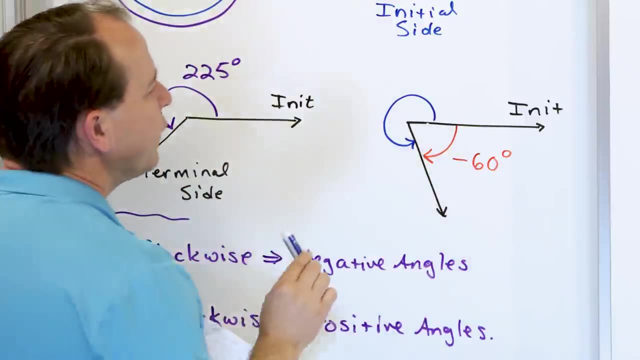 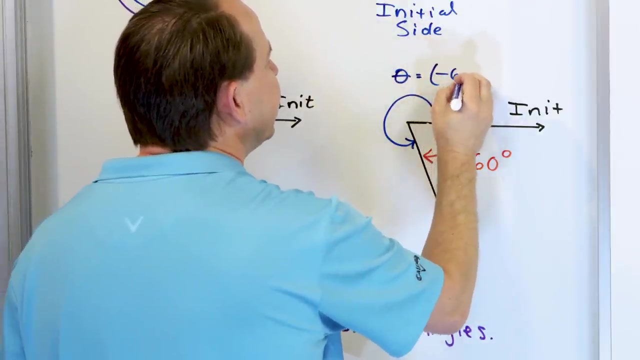 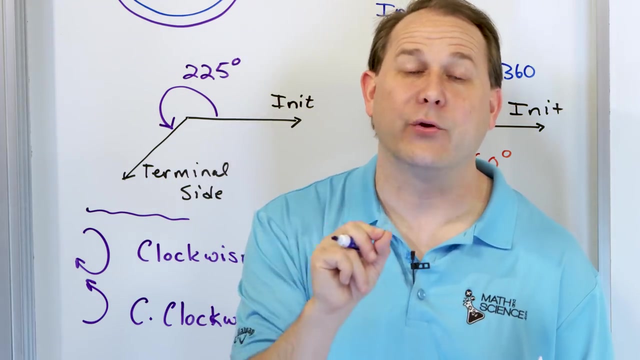 Right, And you know that you can go all the way around the circle and get back to 360 degrees- Right? And you also know that this angle is negative 60 degrees. So what I can do, if I want to define this angle, I'm going to call it theta- I can say that it's the angle I started with- negative 60, and I can add 360 degrees to it, because any angle- this is important- any angle that I add 360 degrees to it just brings me back to the exact same location. 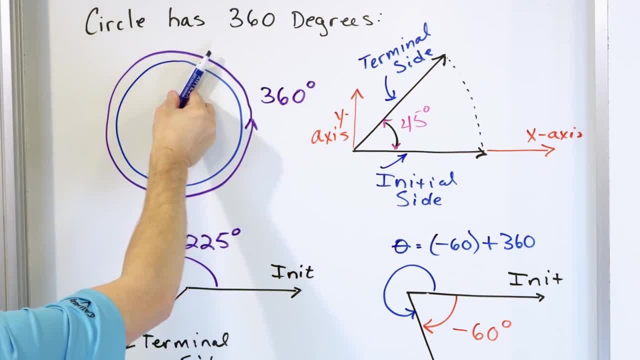 Because, remember, if I start anywhere on the circle, like if I start here and add 360 degrees to that position, I'm going to end up exactly where I started. If I start down here, I'm going to end up exactly where I started. 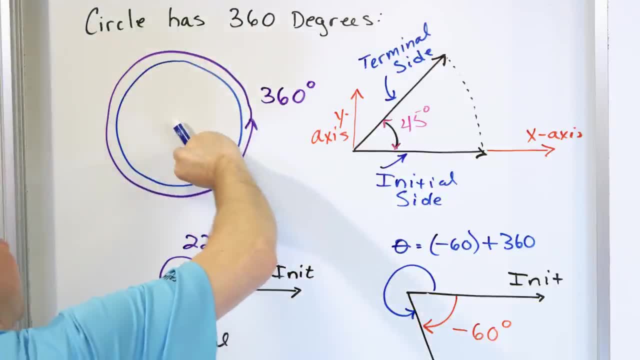 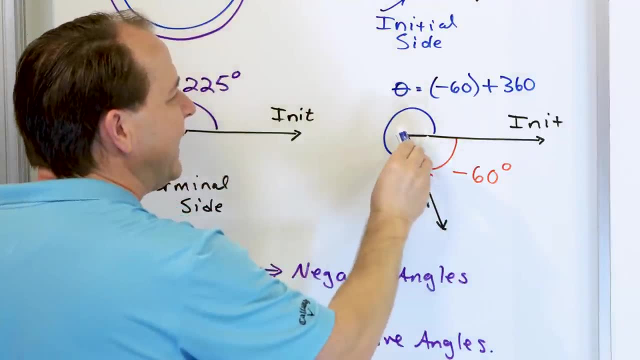 OK, If I start down here and add 360 degrees, I'm going to end up exactly where I started. If I have an angle of negative 60 degrees and I add 360 degrees to it, I'm going to get exactly where I am. 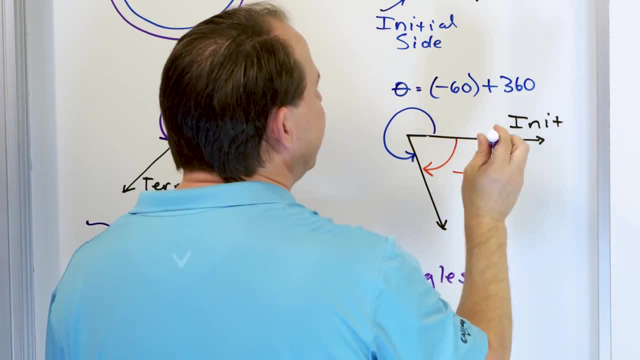 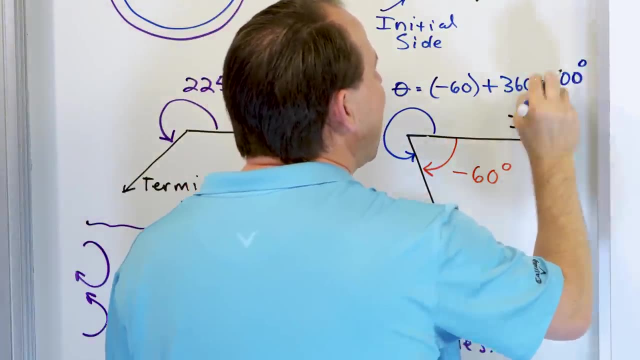 This arrow will be the same, but the angle measure will actually be a positive number. What will this angle be So? negative? 360 plus 60, you might have guessed- is 300, positive 300 degrees. So this angle here can actually be measured two ways. 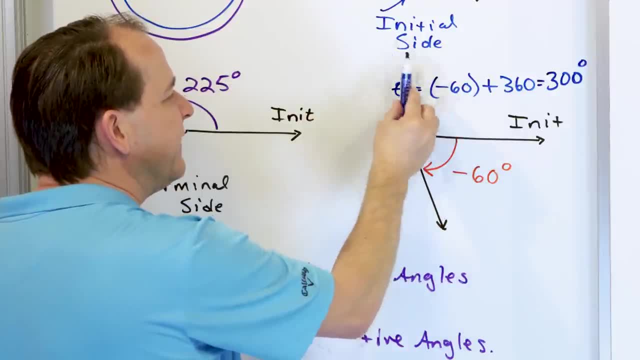 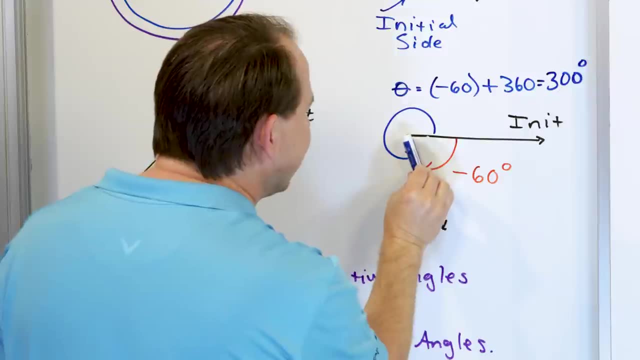 I can measure it as a positive. 300 degrees Makes sense, Right, Because this is 90 degrees, This is 180.. This is 270 degrees going down And just a little bit past. that is going to be 300 degrees. 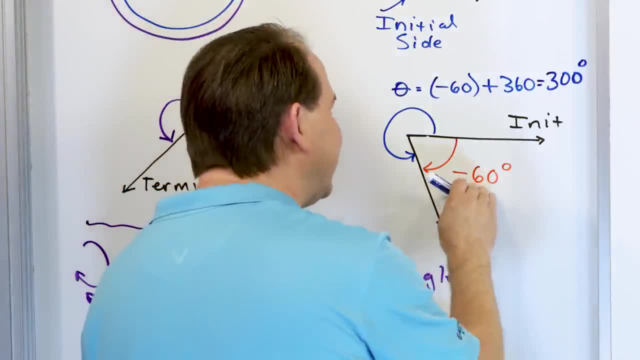 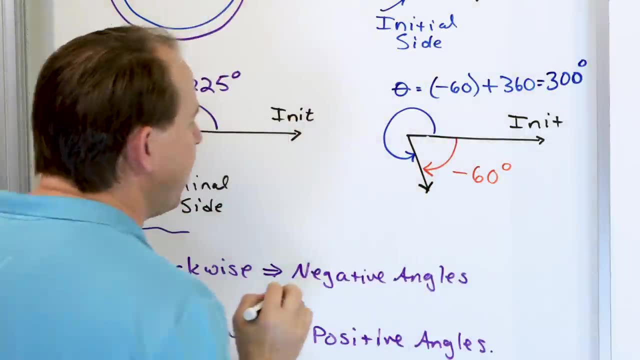 So that's 300 degrees, But it's exactly the same angle measure as negative 60 degrees. So to kind of bring that home, let me shorten this little leg right here, just because the actual length of it doesn't matter, And I'm going to put kind of a nice conclusion down under here. that's really important. 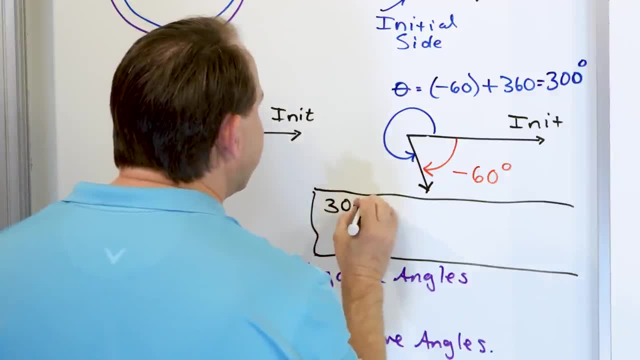 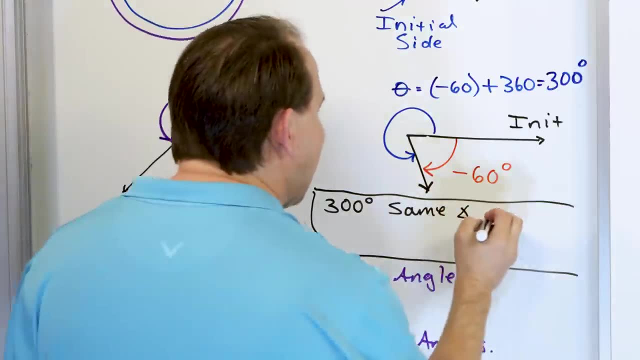 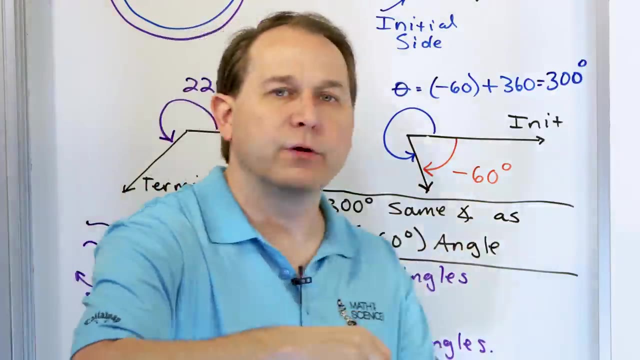 What we're basically saying is that 300, positive 300 degrees is the same angle that this little symbol means angle. the same angle as a negative 60 degree angle. In other words, if I go to the grocery store and tell somebody, hey, I have a 300 degree. 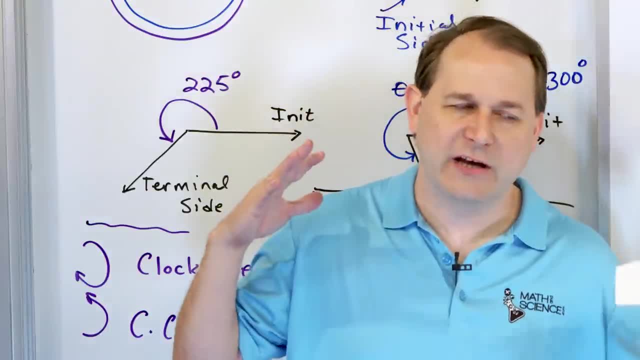 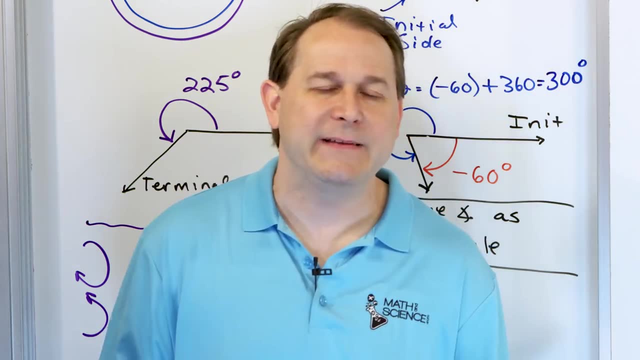 angle. or if I tell somebody: hey, I have a negative 60 degree angle, I'm talking about exactly the same angle, right, Just like five tenths is a fraction And it means exactly the same thing as one half, But that also means exactly the same thing. 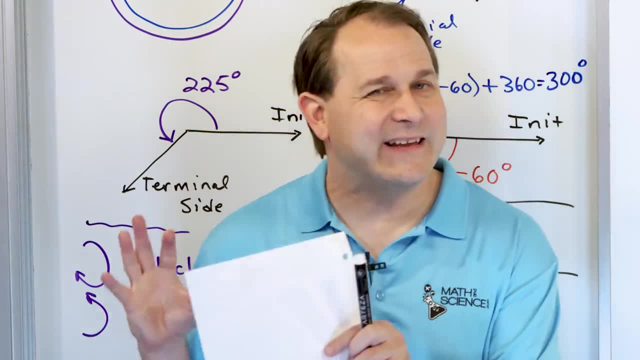 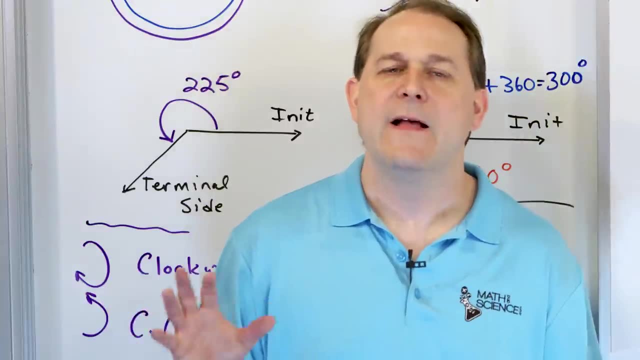 It's exactly the same thing as 50, one hundredths, But that means the same thing as 500, one thousandths. You see the pattern here: Or four eighths, or three sixths, I can go on and on all day. 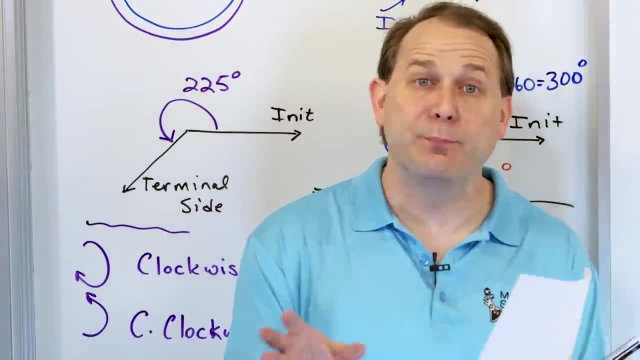 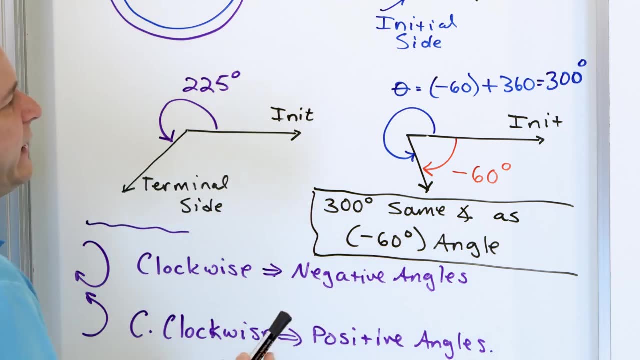 They all mean one half, So angle is the same way. I can have multiple ways of representing the position of this terminal line right here, Some with positive, some with negative angles. In fact, I'll take this opportunity to tell you that of course I started here. I added: 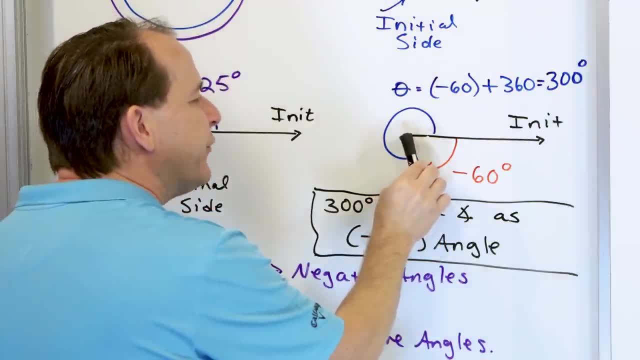 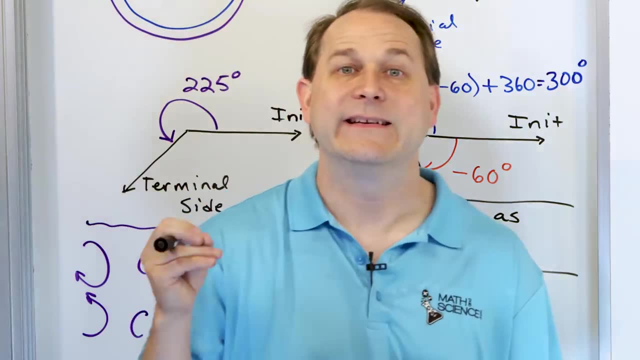 360 degrees to it and I got this angle. What if I add 360 degrees again? I could add 360 degrees to the 300 degree angle. What am I going to get? 660 degrees. So 360 plus the 300 is 660.. 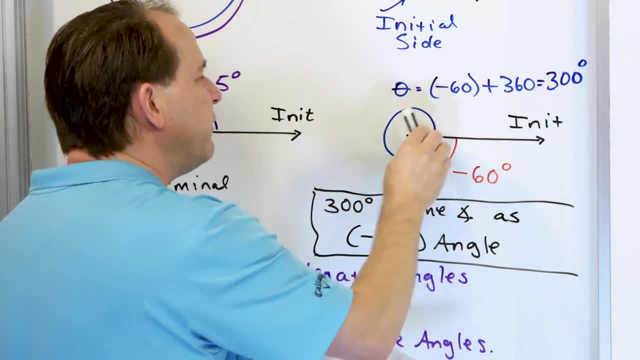 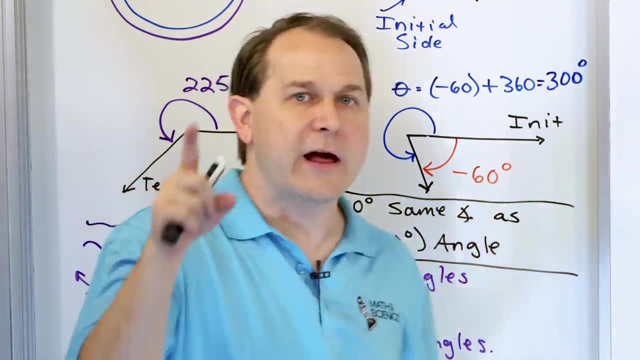 So this angle also could be negative: 60 degrees, It could be 300 degrees. Or if I add 360 again, it could be 660 degrees. I could add another 360 and another 360.. I can keep doing this forever. 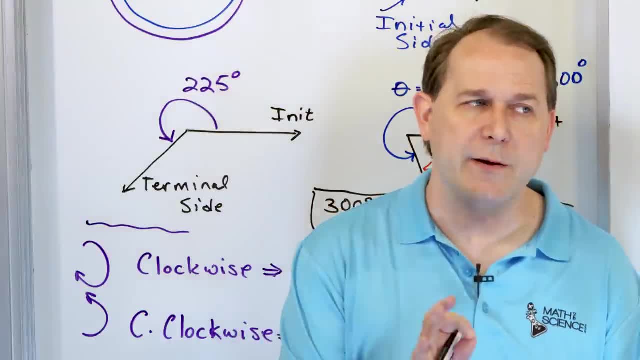 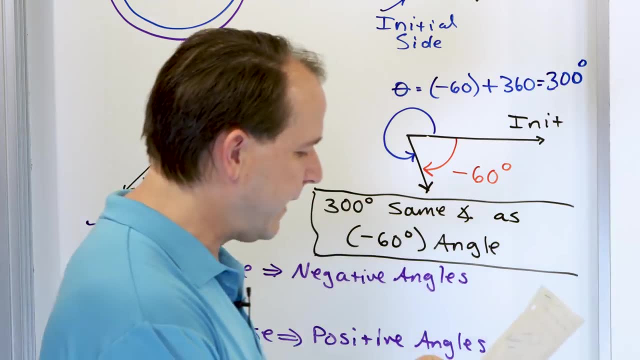 And I can come up with many, many, many, an infinite number of angles, measurements that actually correspond to exactly the same thing. You have to kind of get used to that when we talk about this. So we talked about angles, how they're measured- positive angles, negative angles. 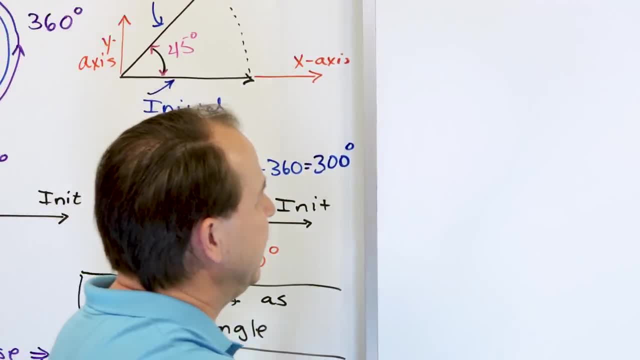 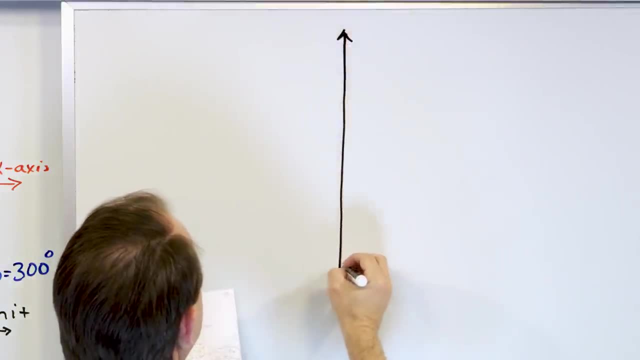 Now we need to talk about quadrants, quadrants of the xy-plane, Because you're going to be asked to be talking about the quadrants where these angles kind of exist in the xy-plane. So we'll talk about a couple right here. 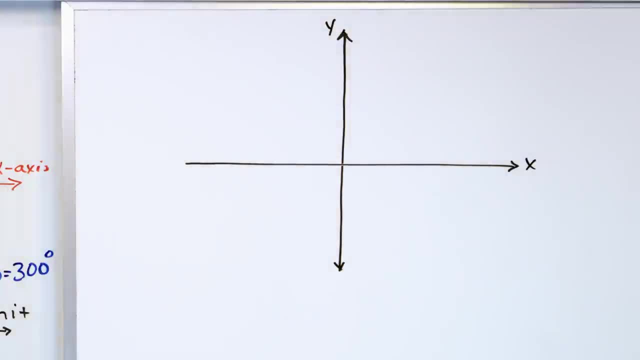 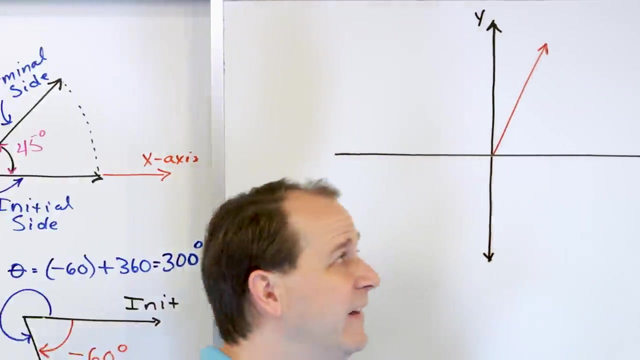 So this is the x-axis, This is the y-axis, All right, So let's take a look at an angle that exists. let's say, right here, Now: every angle has to have an initial side and a terminal side. The initial side. from now on, unless I tell you otherwise, the initial side is always. 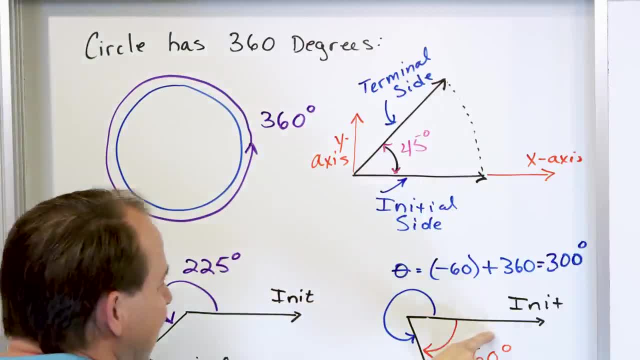 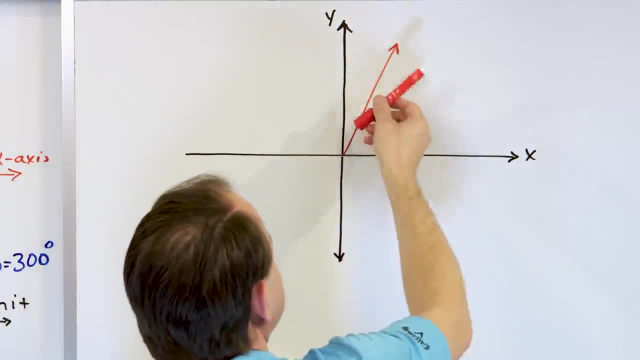 going to be the x-axis. The initial side is the x-axis. The initial side is the x-axis. Even here I kind of didn't draw it, but the initial side was the x-axis right there. So the angle that defines this guy right here starts from here and ends right here. 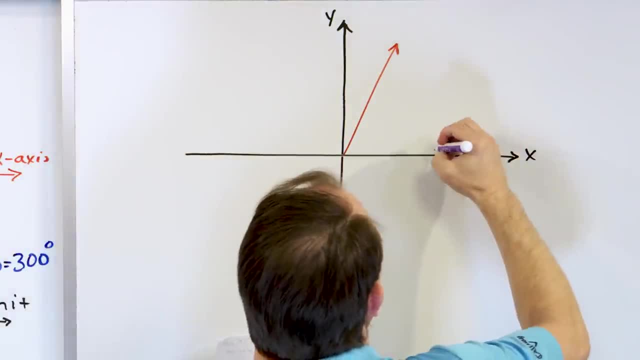 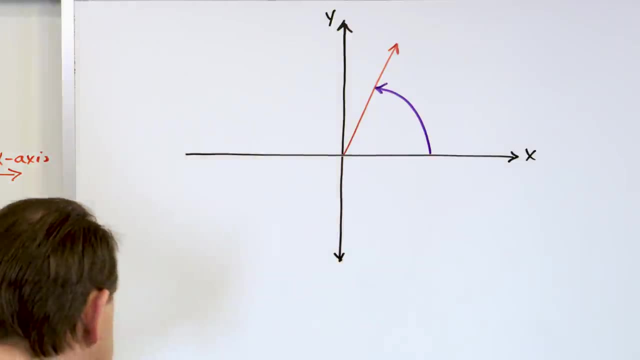 So you could say that that angle goes, That angle goes up, something like this: I could draw it really close if I want to, or I could draw it far away, It doesn't matter, As long as I start somewhere and end somewhere. that angle can be defined like this: 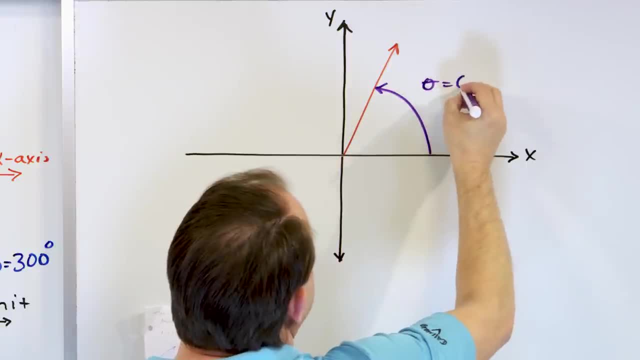 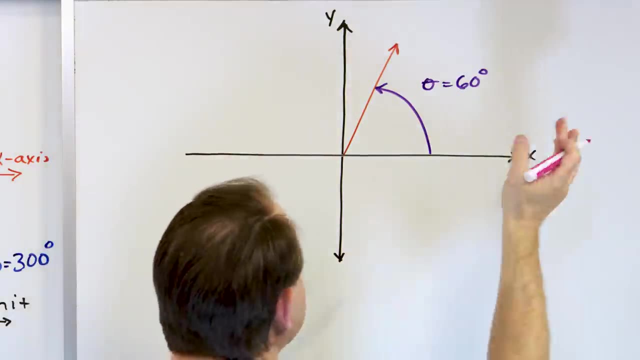 What is this angle? Well, I'm going to tell you that this angle is 60 degrees. Now you have to go back and think about quadrants. We talked about quadrants a long time ago. This is quadrant number one. This one over here is quadrant number two. 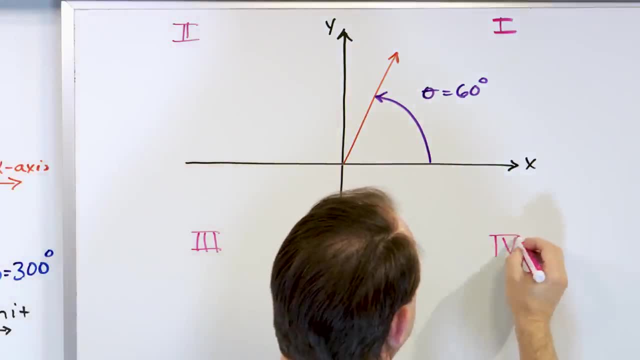 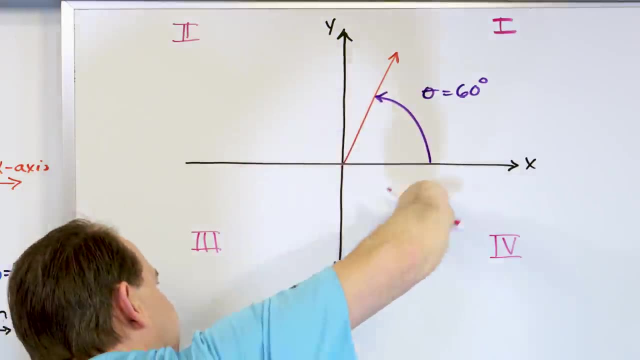 This one over here is quadrant three And then this one over here is quadrant four. So it goes, the same measurement, the same direction of positive angle measures goes quadrant one, quadrant two, quadrant three, quadrant four, like this. So if I asked you what quadrant is this angle in, then it would be a simple answer. 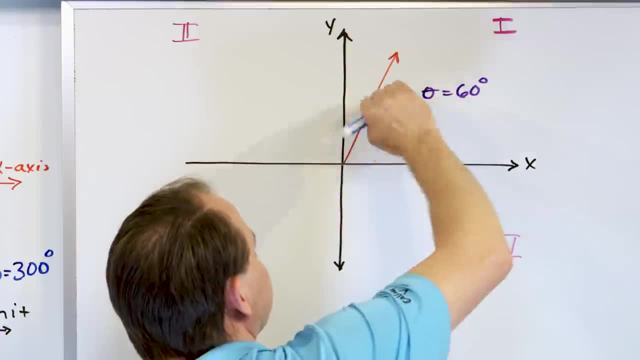 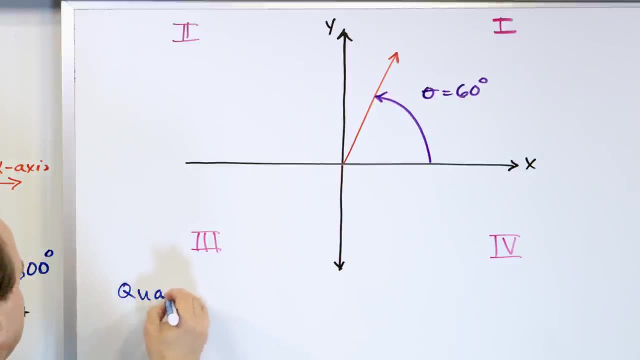 You would say: well, the A-terminal line here, this is the initial and this is the terminal. The terminal part of the angle is in quadrant one. So we say this is quadrant one angle, Because you're going to have some problems. that'll basically say, let me know what quadrant. 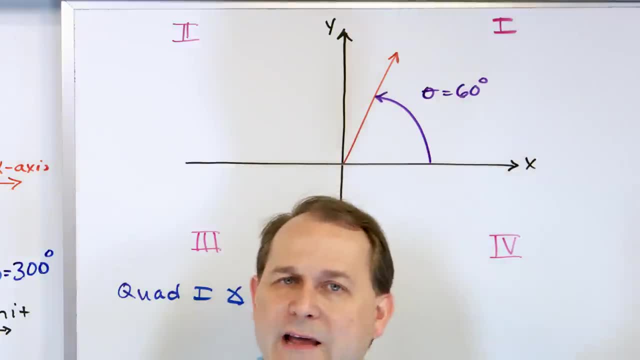 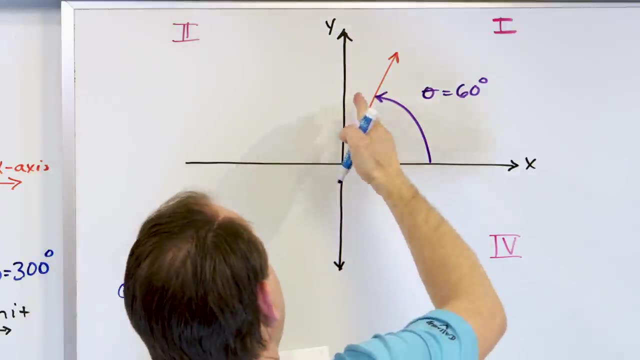 this angle is in. All you do is look and see where the line, the terminal line of the angle, falls. That's the quadrant it's in. But we'd said that all angles can be measured positively or they could be negative measures. How would you measure this angle in a negative fashion? 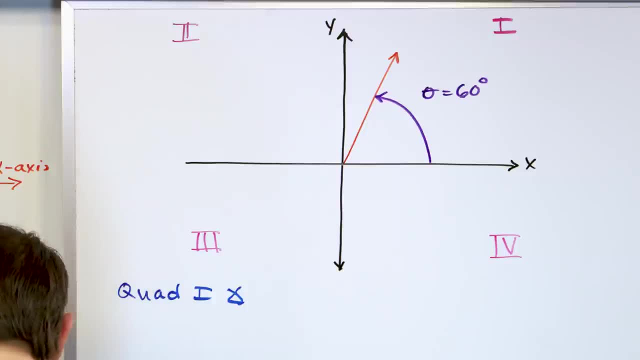 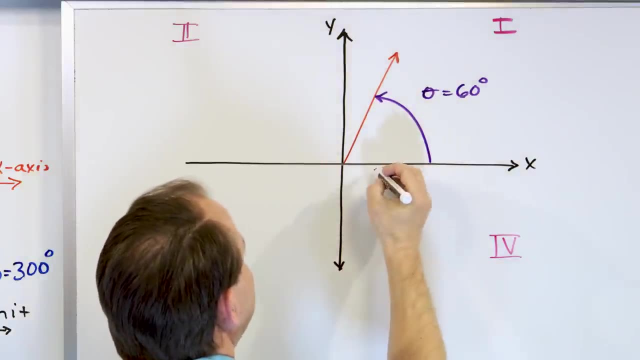 If I were to measure this angle in a negative fashion, I'm just going to get the right color, Let's use this one. If I measure this angle in a negative fashion, I would have to start again at the X-axis, but I would have to go the other direction, all the way back to here. 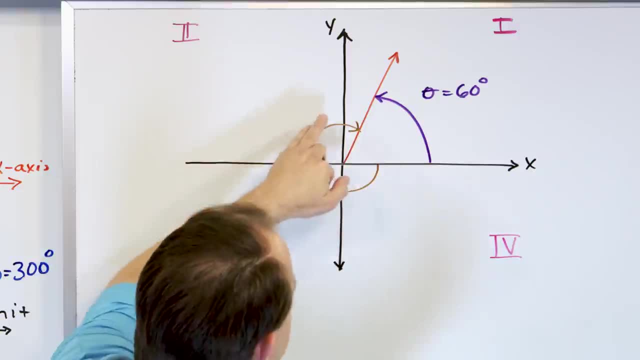 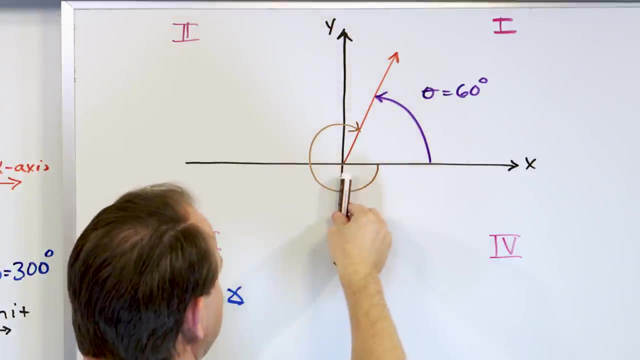 Like this, And this angle would not be a positive angle, it would be a negative angle because it's measured down going below in a clockwise fashion like that. How can I figure out what this angle measure is? Well, this is negative: 90 degrees. 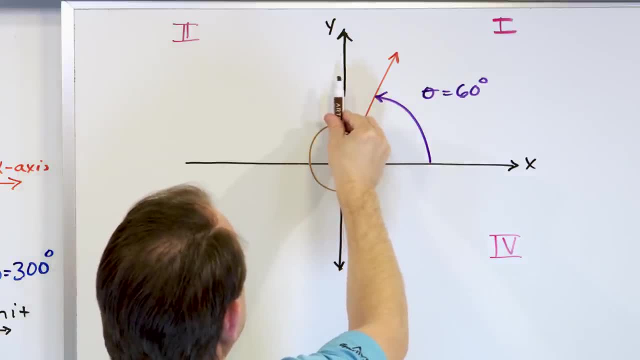 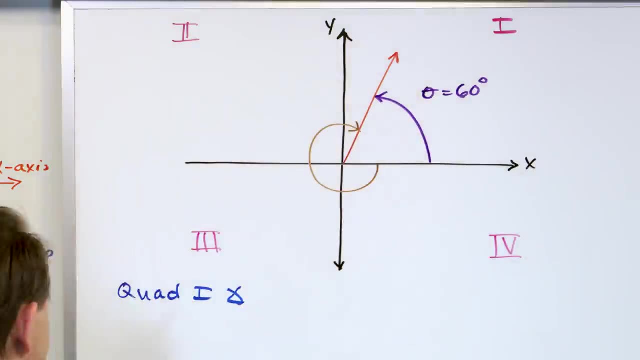 This is negative 180 degrees. This is negative 270 degrees And this is just a little bit more than that, And since you know that this is 60 and you know that this is another 90, you could probably guess what this angle is. 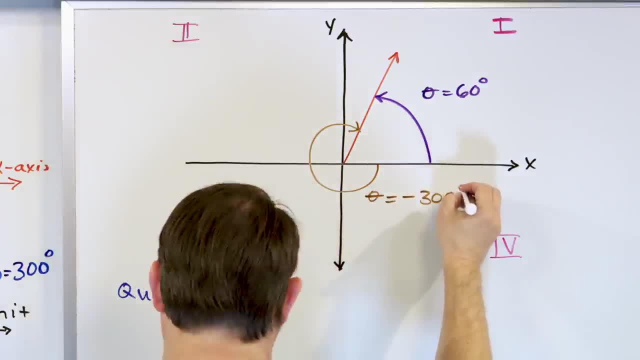 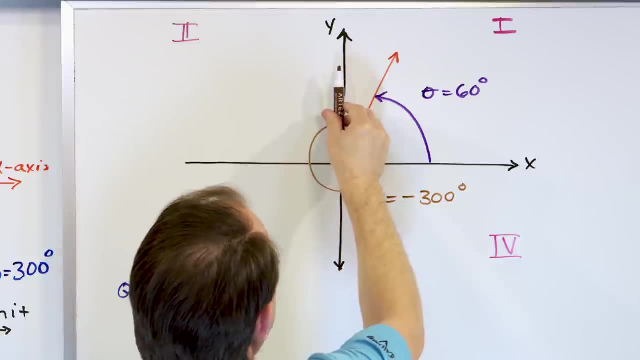 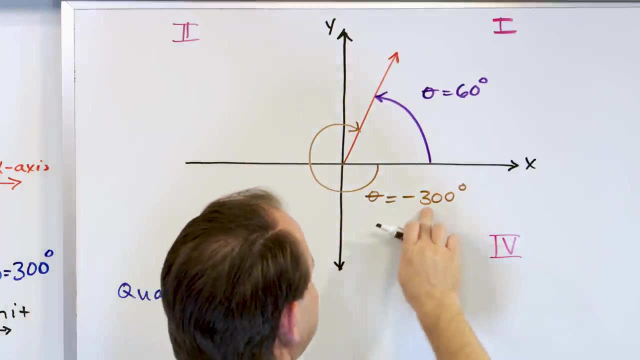 This angle is negative 300 degrees, Negative 300 degrees. So what's negative 300?? Because this is negative 90,, negative 180,, negative 270, and this has to be 30 more. Because this is 60, and 30 and 60 is 90,, it has to be 30 more from 270, so it has to be. 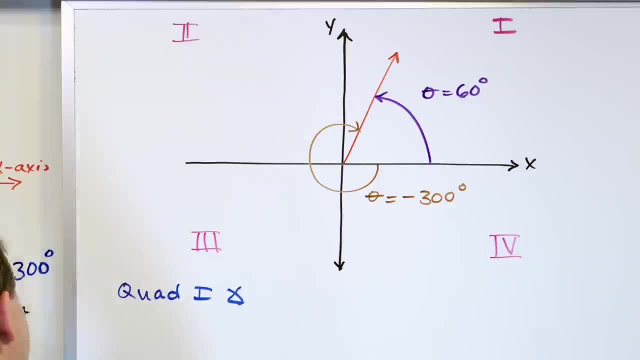 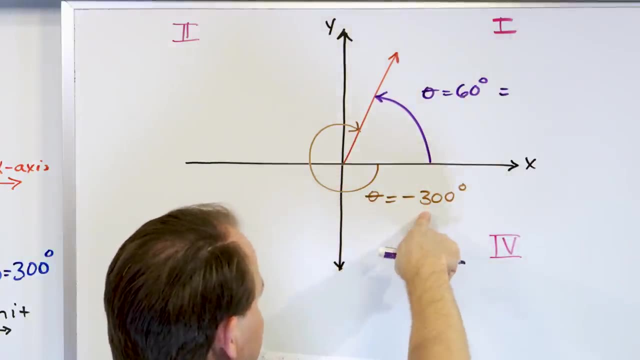 a negative 300. So another way to say that I mean we kind of talked through it and that's all great. How do we figure this out mathematically? Well, if I take the angle that I think that it is negative 300, and I add 360 degrees, 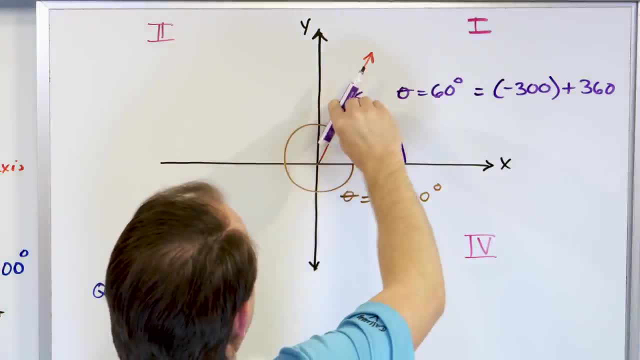 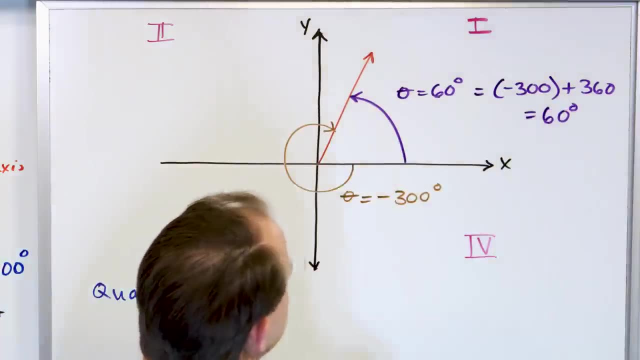 to it. I think it's negative 300.. I'm going to add 360 degrees to it, so I'm going to spin all the way back around to where I started, and then what I'm going to get is positive 60 degrees. 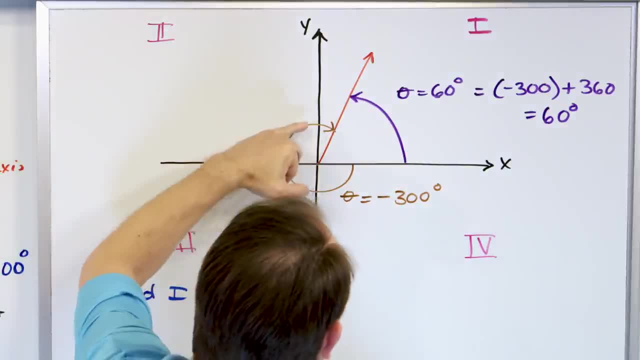 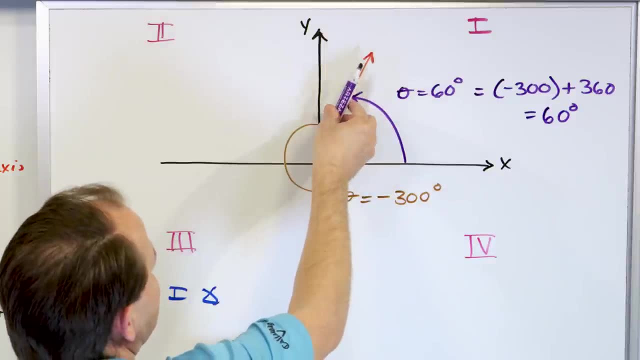 So another way of saying this is: I know that this angle measure is also negative 300, because if it is negative 300, then that tells me where this is, And if I add 360 degrees to it and I'm going to spin all the way back around to where I? 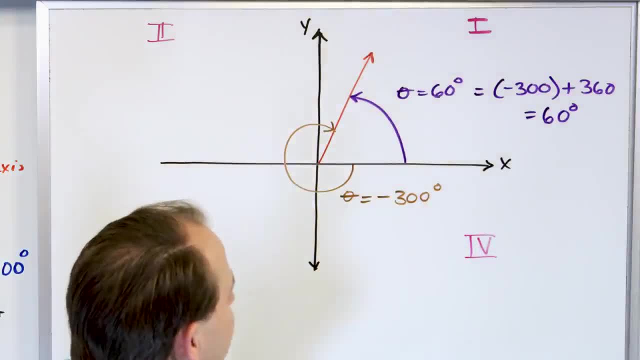 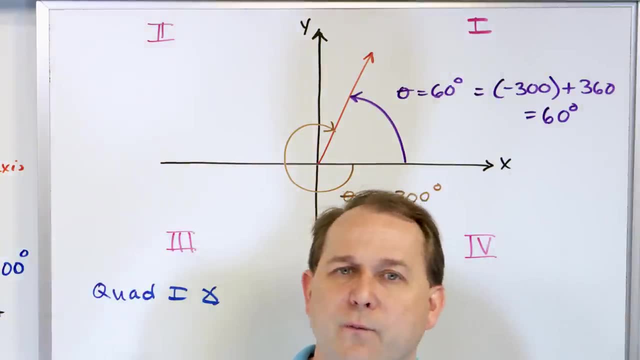 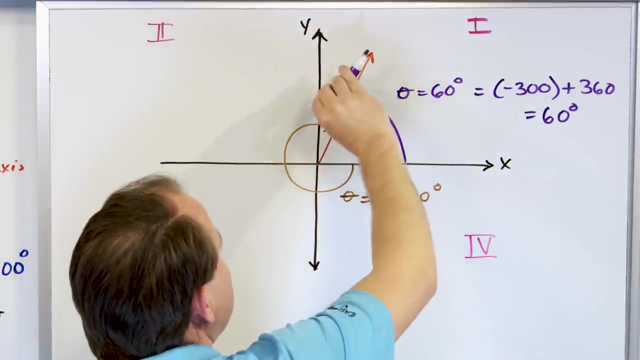 start and I'm going to get a positive 60 degree angle. So this angle is 60 degrees positive or negative, 300 degrees negative. Those are just two of infinite number of ways to write this angle Because, again, if I know that this angle can be expressed as 60, I can add 360 again. 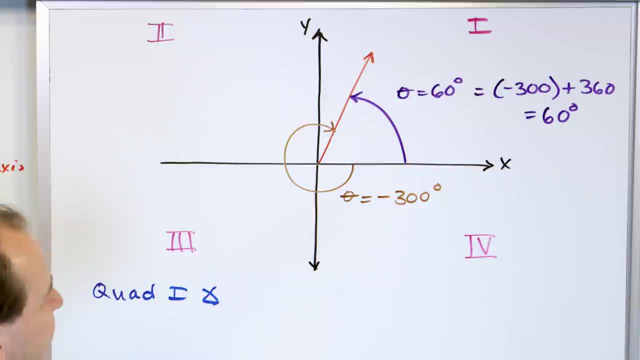 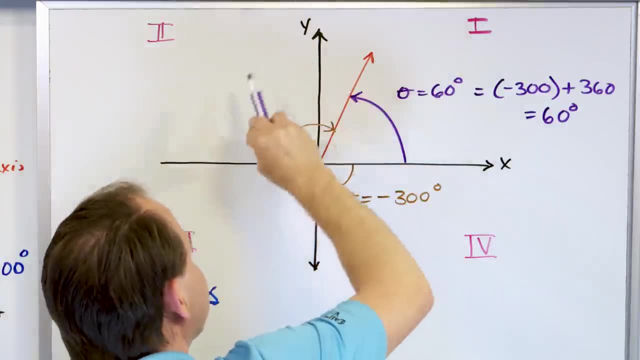 What am I going to get? 360 plus, uh, 360 plus 360. That would be another 360 plus 60 degrees would be another angle measure, And then I can add another 360 and another 360, or whatever. 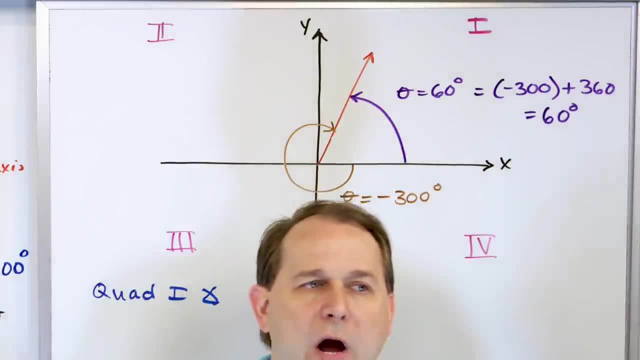 In other words, I can add and subtract 360 degrees to angles. all I want and continue to get new angle measurements that are telling me the exact same information. Where is the terminal end of that angle? That's all. that's all I care about. 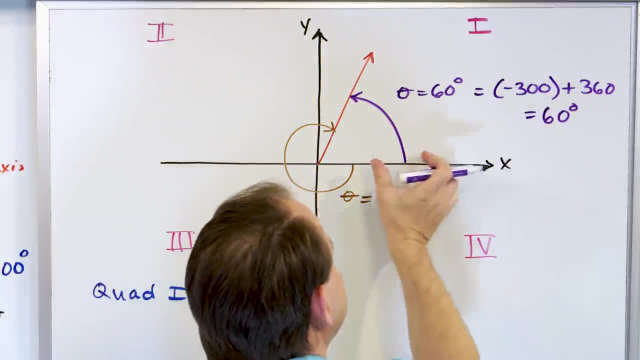 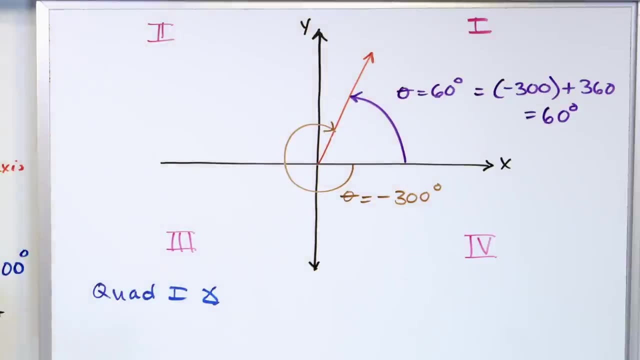 Okay, But the point is is no matter if this is a positive 60 degree angle measure or if it's a negative 300 degree measure. the terminal side here is still in quadrant one. So it's a quadrant one angle. That's all that matters to these kinds of problems. 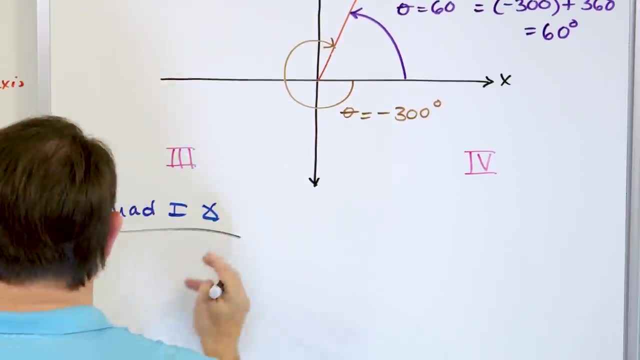 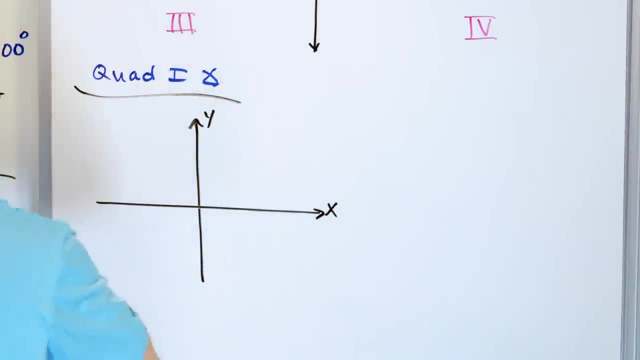 Okay. So to bring that point home a little bit more, let's do another one. Let's say: I'm going to have an angle measure. that's a little bit easier to understand. Let's say X and Y. Let's go ahead and draw another angle measure in here and let's draw it over, something like: 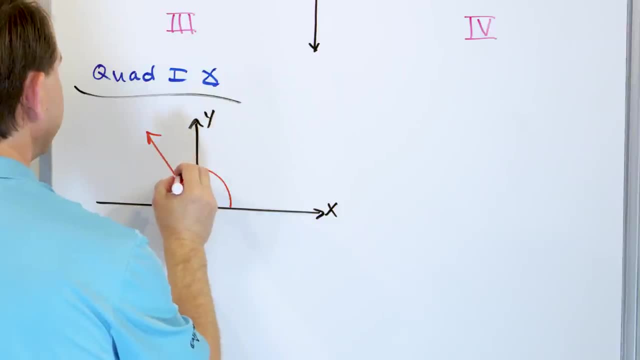 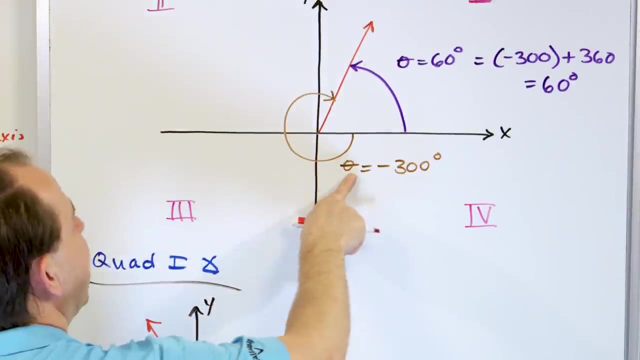 this, And let's say that this angle, starting here, measured in the positive direction, is 120.. And, by the way, I keep using this: angle theta, angle theta. uh, used it here. angle theta. I probably wrote it down somewhere over here. 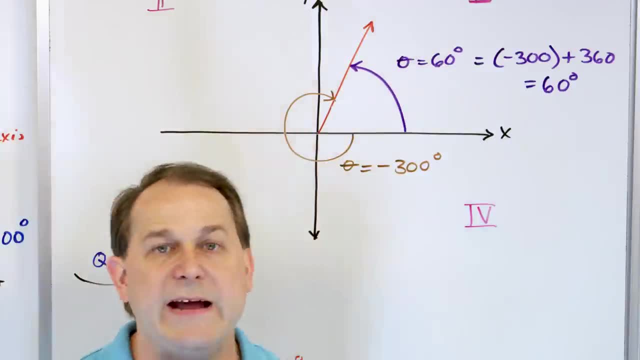 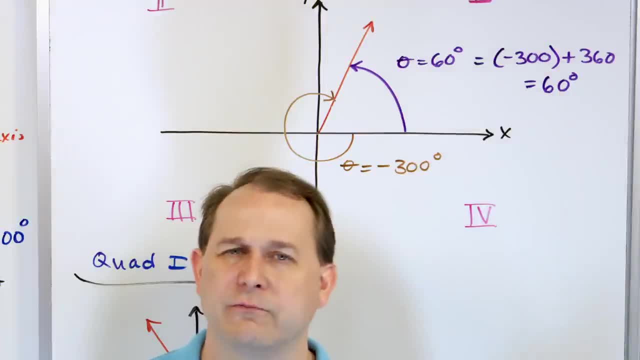 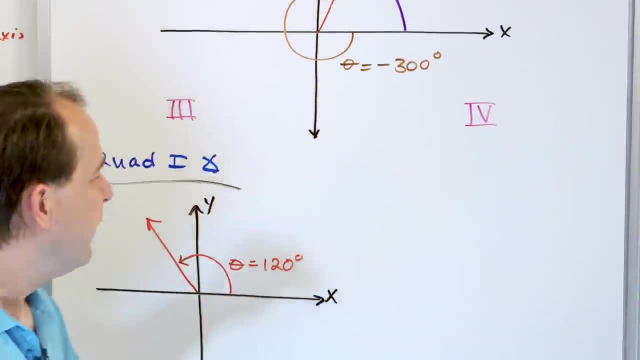 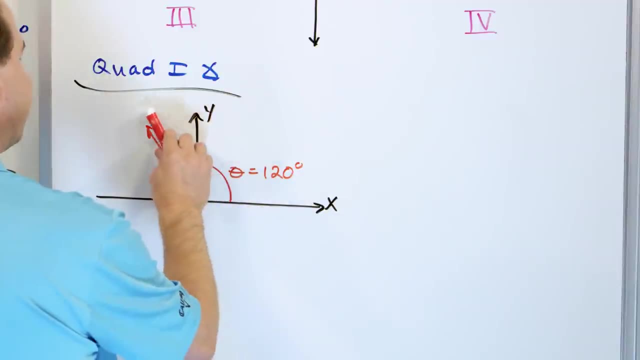 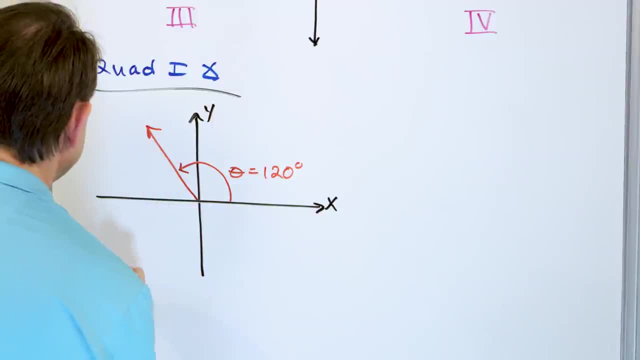 So what quadrant is this angle in? This is the second quadrant. Okay, If I take this and I add or subtract 360 degrees to it, I will get different angle measures, some positive, some negative, but it's still expressing where this is in quadrant two. 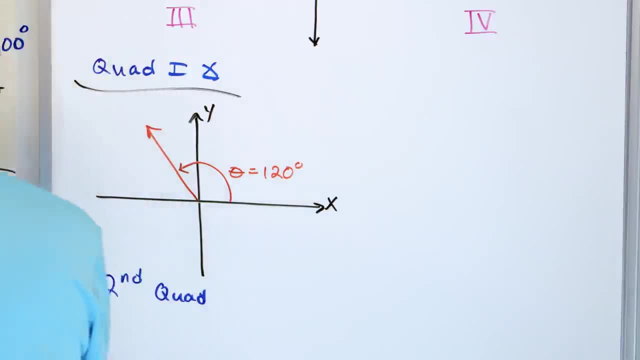 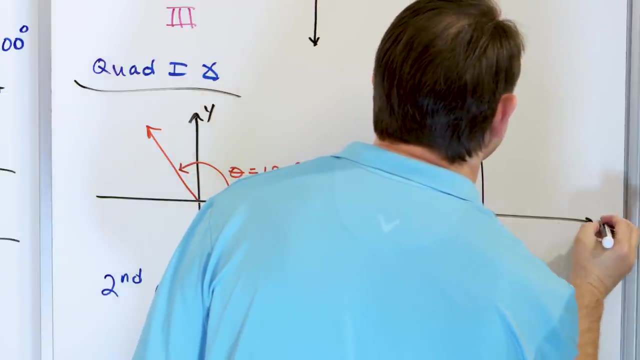 So it's a second quadrant angle. okay, Let's take a look at another one. This one's actually a little bit more interesting. What if X and Y like this? what if my angle is? what do I wanna draw it here? 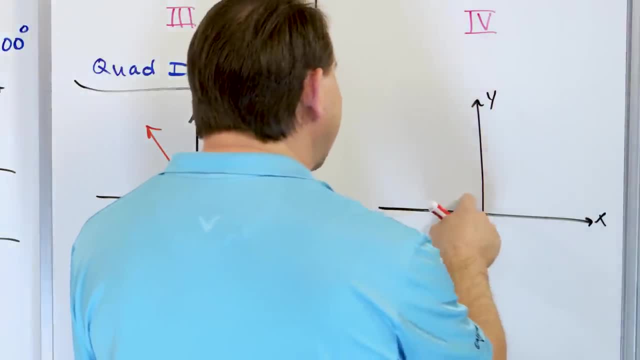 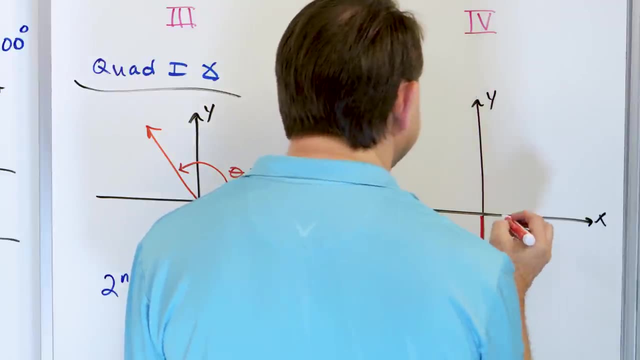 Down here. What if the angle is not exactly over here or over here, or over here or over here? but what if the angle is basically right on top of one of the axis, like this, So the angle measure going all the way around here? 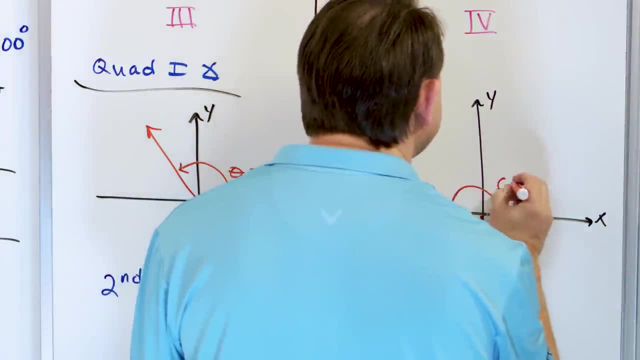 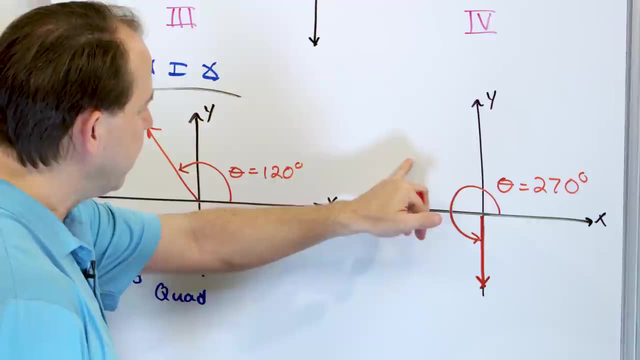 this is 90,, this is 180,, this is 270.. So this angle is 270 degrees. What quadrant does it fall into? Well, it's not the first quadrant, It's not the second quadrant, And it's not in the third or in the fourth quadrant. 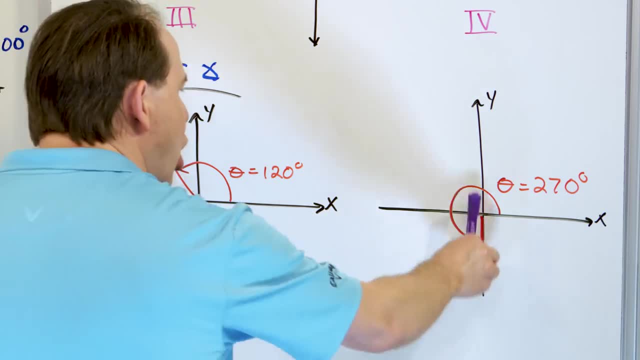 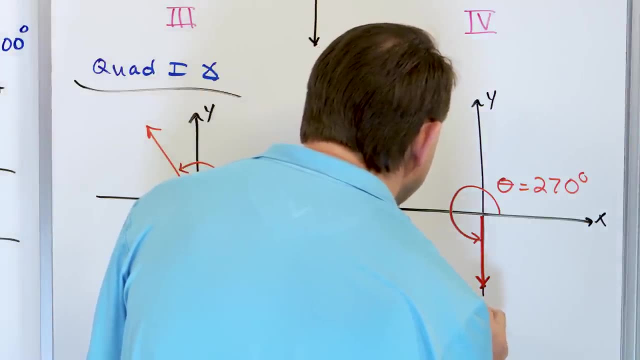 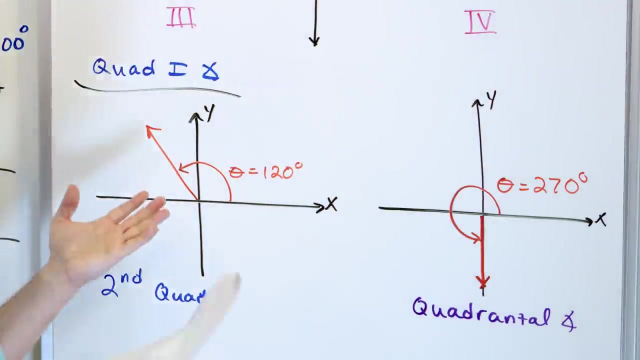 It's right in the middle. If one of the angle measures falls right on one of these these lines right here, it's not in any of those quadrants, It's just called a quadrantal angle, Quadrantal angle, okay. So the bottom line is you'll be asked some questions. 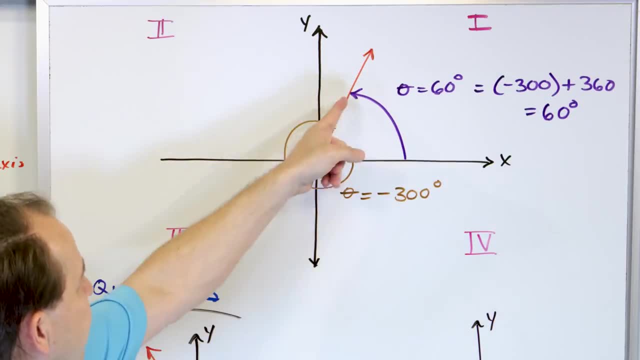 Here's an angle. Tell me what quadrant it's in And you just have to look and see where it falls. If the angle falls over here, it's in the third quadrant. If the angle falls over here, it's in the fourth quadrant. 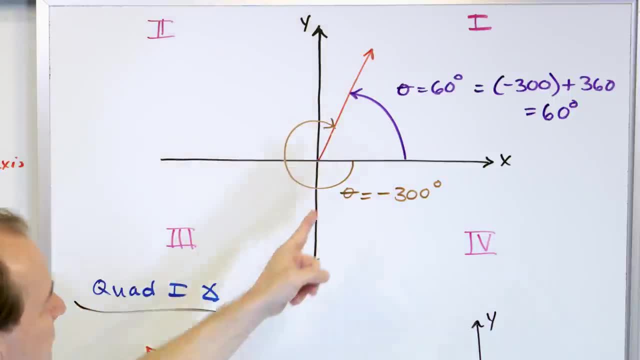 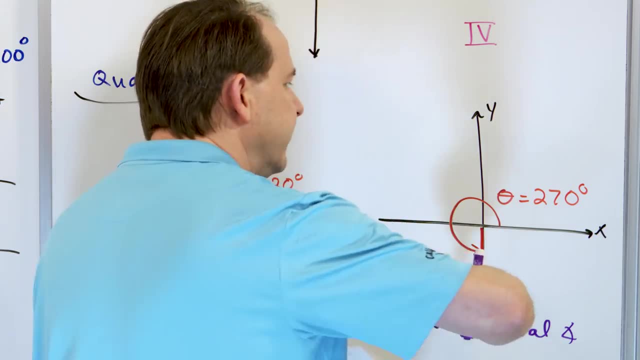 If the angle's over here, it's the second quadrant. like this one, Angles over here are in the first quadrant If the angle falls on this line or on this line, or on this line or on this line, in other words, zero, 90,, 180,, 270,. 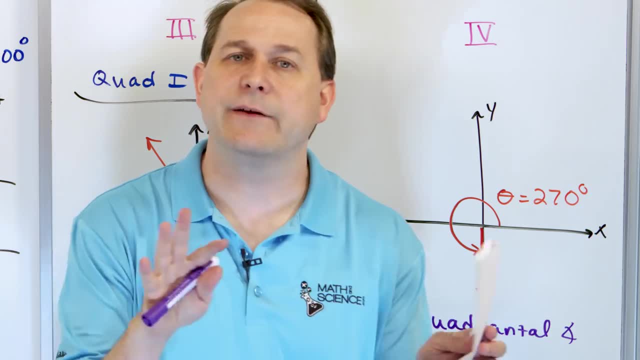 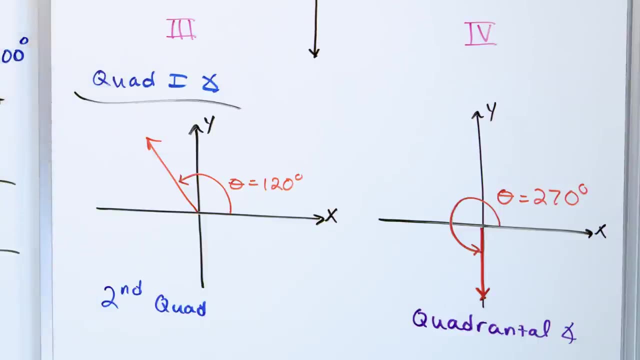 or even back around to 360 degrees, then it's not in any of those quadrants. We just say it's a quadrantal angle. That's all that we say. All right, now we have gotten at least about halfway through this lesson. 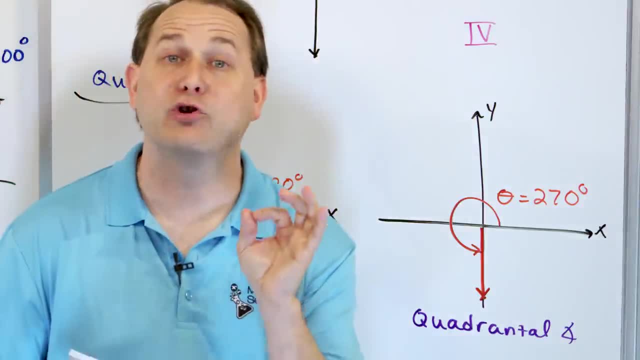 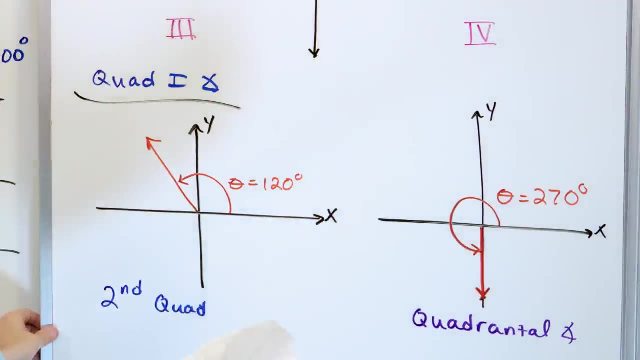 We've learned the most important concepts, but we have one more thing to talk about. We have to talk about coterminal angles. It has a fancy-sounding name, but I've actually already taught you kind of what coterm terminal angles really are. 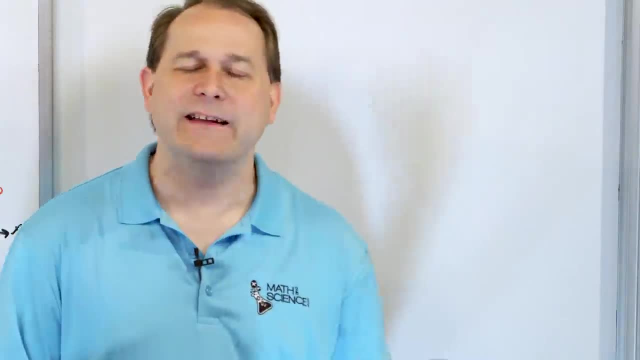 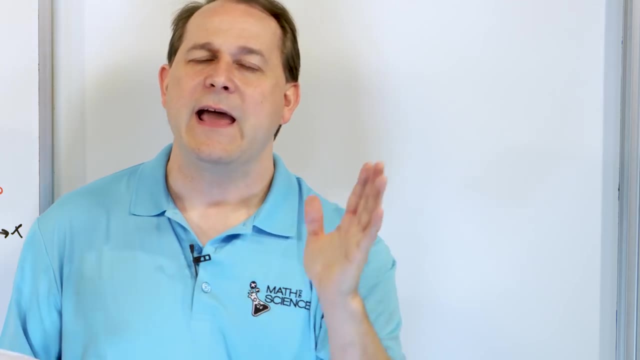 Coterminal angle just means that I can add and subtract 360 degrees to any angle I want, and I'm going to get another angle that is exactly kind of in the same position, And so those angles are kind of equivalent as far as like where they're at. 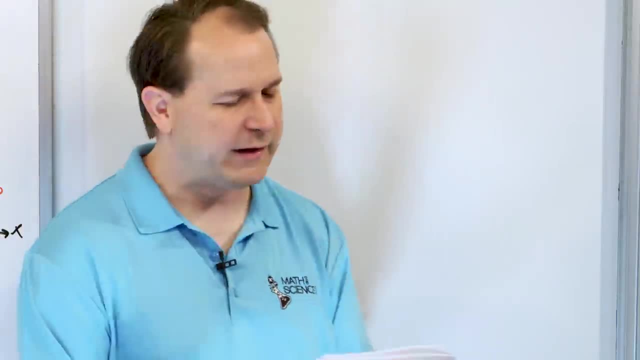 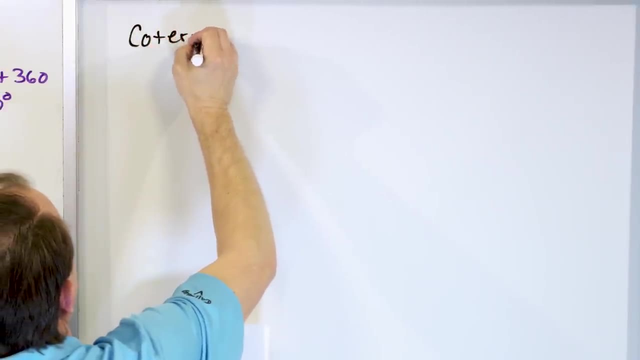 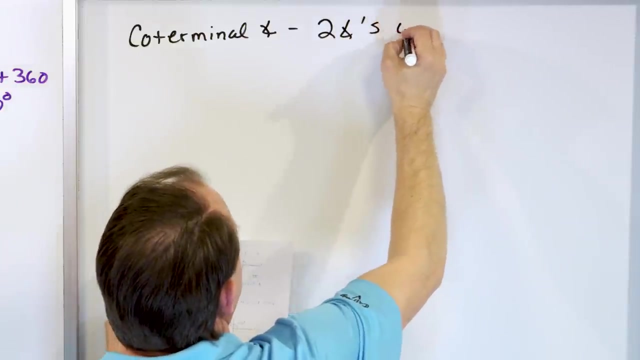 They have the same terminal point, so we call them coterminal, That's all it is, And so let's talk about that. It's a definition you'll need to know. Coterminal, Coterminal angle, And these are two angles where terminal. 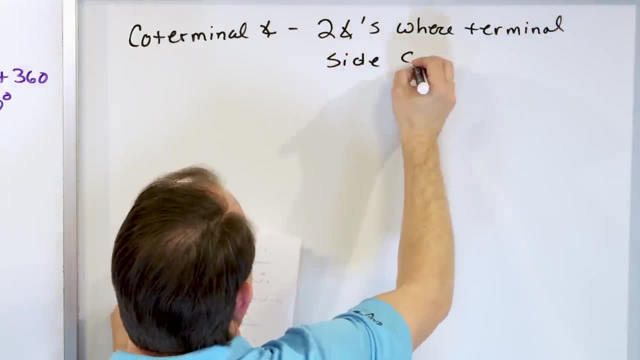 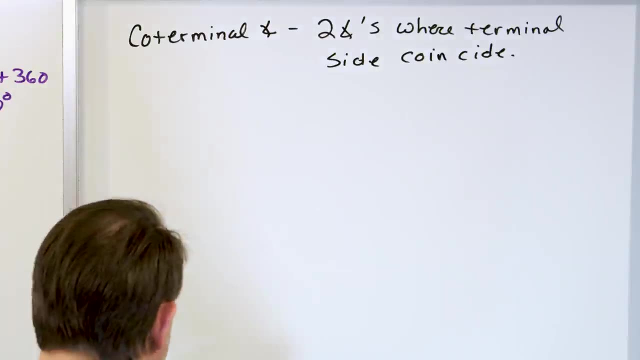 side coincide All right, and we've kind of done a lot of these over here, so it's not gonna be a huge surprise what we have here. but let's take it one step at a time. We're gonna draw four pictures. 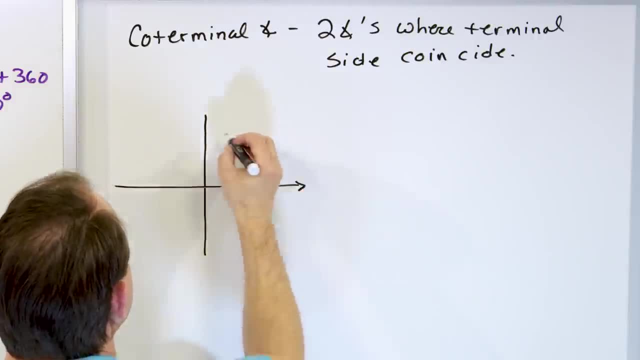 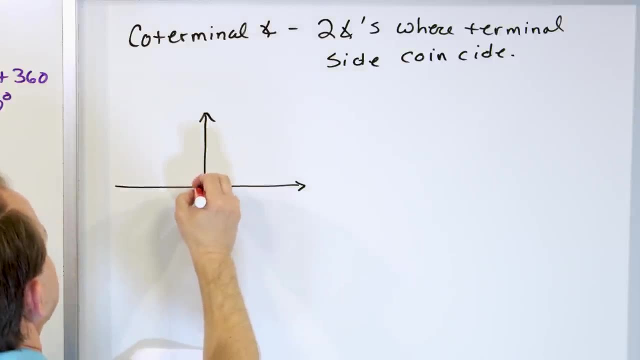 I'm gonna try to keep them all on the same board and try not to keep them too large, so I can make sure that you can see them all. All right, have the first angle goes off like this and the angle here is 150 degrees. okay, First of all, 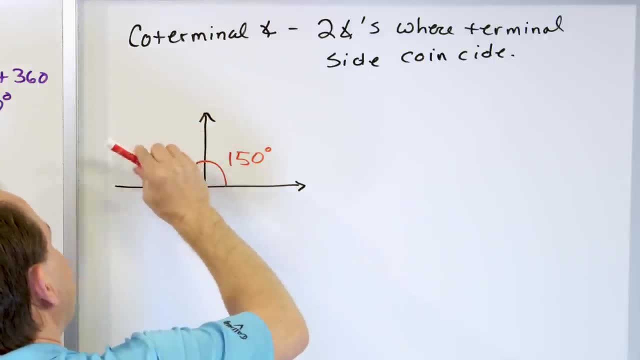 what quadrant is that angle in? Well, this is quadrant one, this is quadrant two. so this is a second quadrant angle. It's a positive angle measure because we're measuring counterclockwise, like this: This is 90,, this is 180, so we're not quite to 180, so this is 150.. It makes sense. 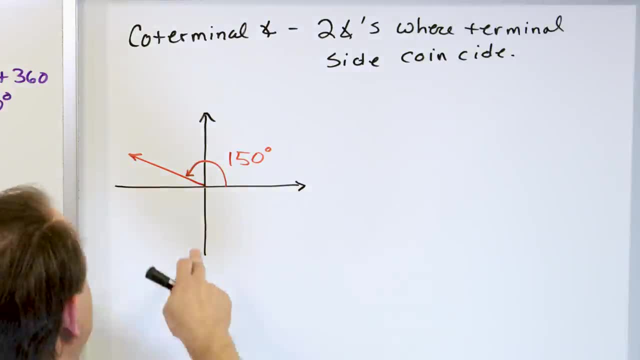 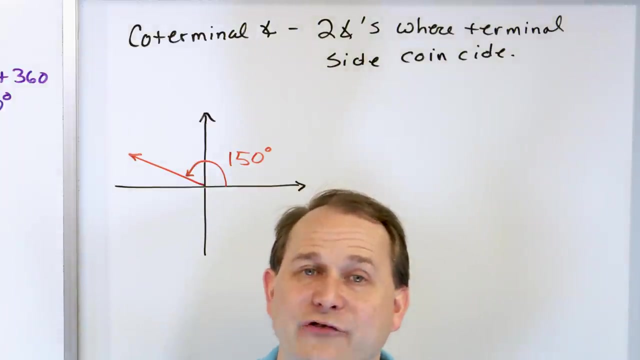 okay, Now what's going to happen if we add 360 degrees to this angle? We just said, if this angle measure is here, we can add 360 by just sweeping around a full circle from that and landing exactly where we start. It's going to express the same location of that terminal side. that's why it's. 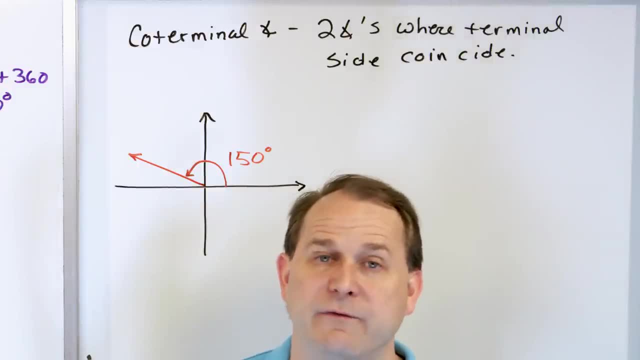 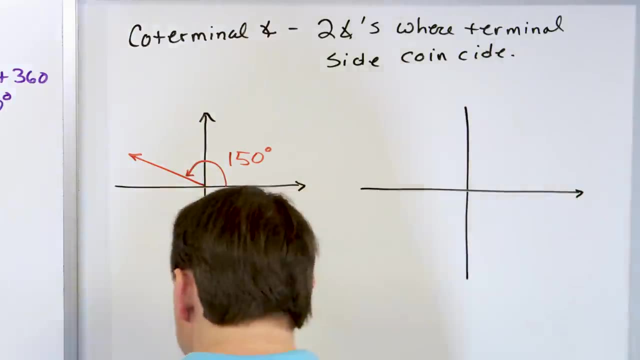 called coterminal, but the angle measure will be bigger than 150 because we're adding 360 to it. So this is what it looks like. okay, The coterminal measure will be bigger than 150 because we're adding 360 to it. 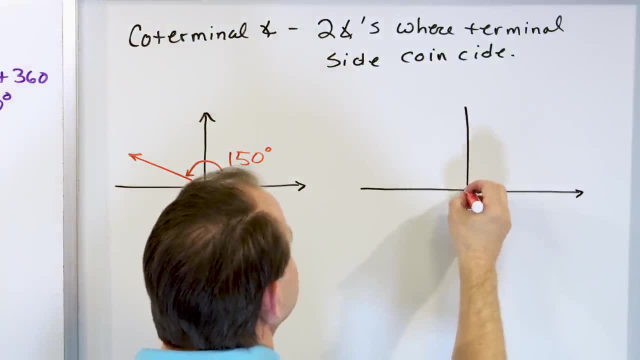 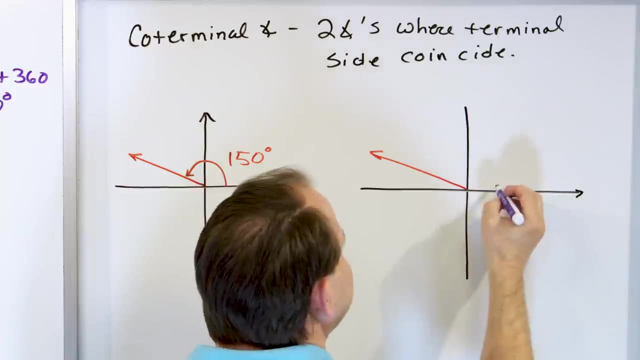 The coterminal side is exactly in the same position. so I'm going to do my best to draw more or less the same exact thing. but here's the weird thing: What we do is we start at the same initial side, we go all the way to 150, but then we go right through it and continue another. 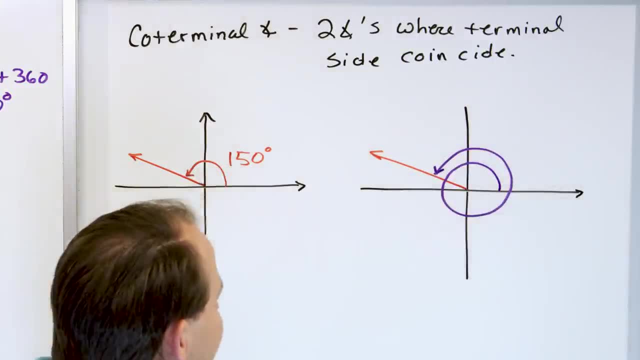 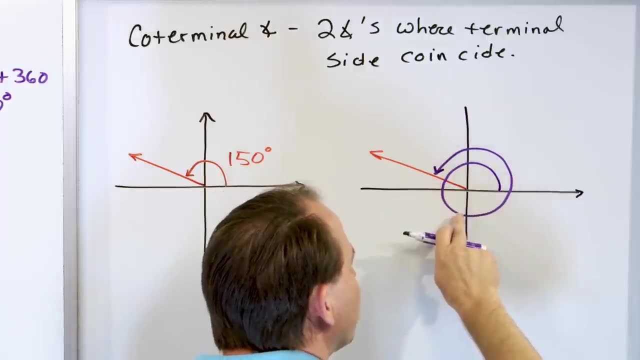 360 degrees landing on that terminal side. So if you think about it from here to here, is the 150,. but then we add- remember the line continued on around in a kind of in a spiral the way we drew it- another 360 degrees landing on that terminal side. So if you think about it from here to here, 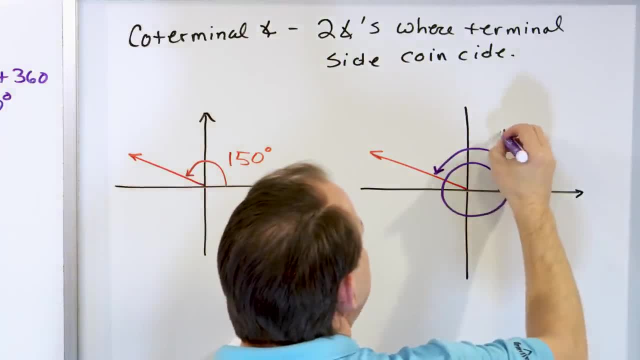 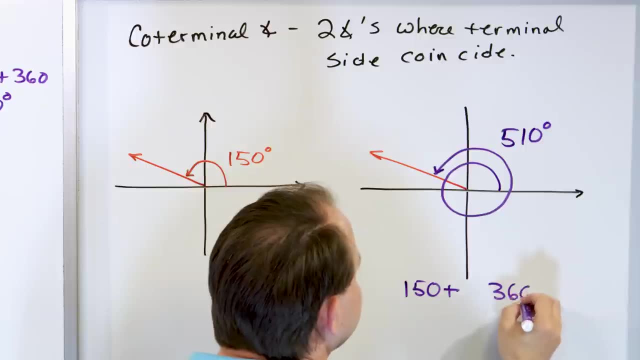 is the same exact thing. So here's the weird thing: What we do is we start at the same exact thing, another 150 degrees landing on that terminal, but then we go right through it and continue another 360 degrees landing on that terminal side. So let's just say, okay, up to where is my? 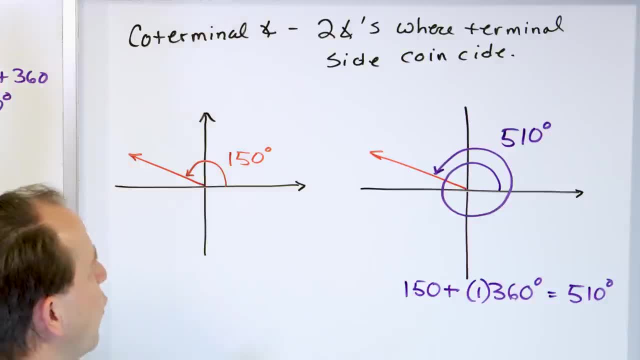 base point of gray And I'm going to say a little bit higher. So if you just look at this here, your base point will change mixed, since as you have to drag the angle up just a little bit, when you have to drag the angle up just a little bit, bear in mind- I think this is another- 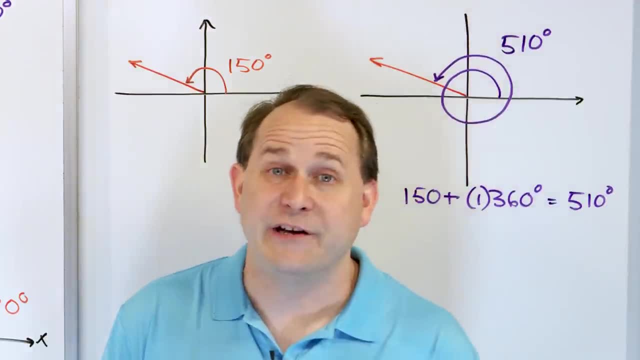 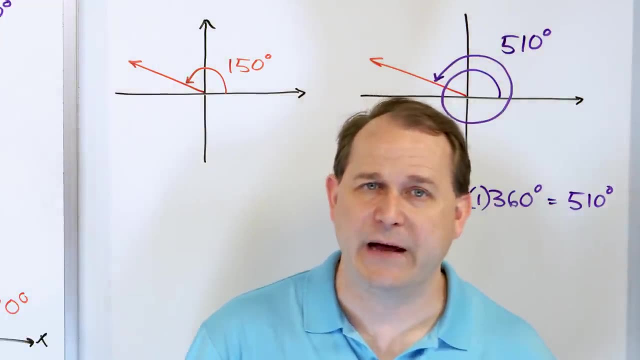 będzie gak разные square drink. You might not be familiar with colorulations of color in dual. we're kind of building the foundation here. We know that we're not gonna express 510 degree angles very often, but you need to know that it is exactly the same thing. 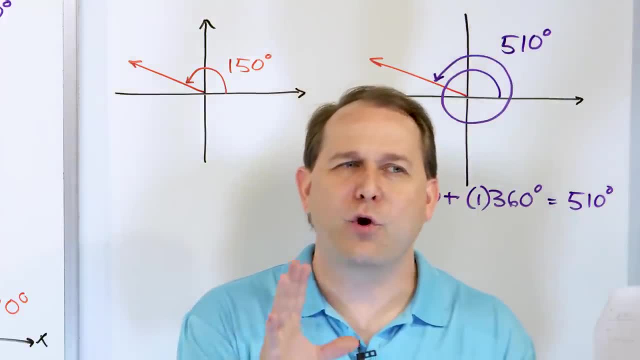 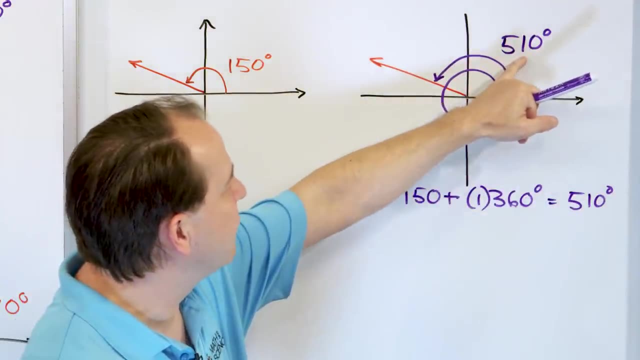 Because sometimes, when you're solving equations, you get large angles, but then you don't wanna it's like a fraction, you wanna simplify it to the kind of the smallest number you can, And so you would need to know if I got 510,. 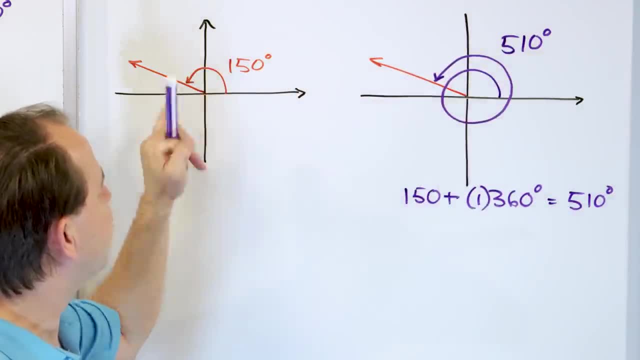 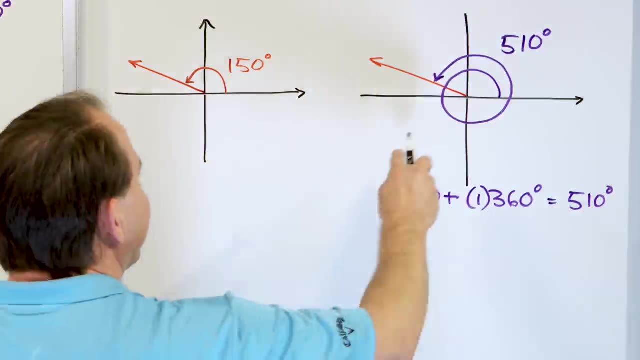 I'm just gonna subtract 360 from it and I'm gonna get the smaller angle that still expresses the exact same thing. Okay, now we don't have to stop there. We can, of course, add 360 degrees again if we want to. 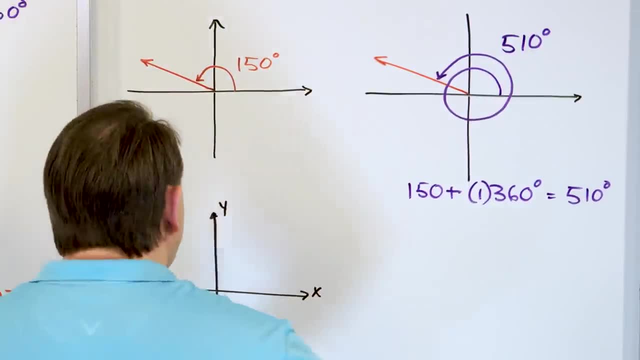 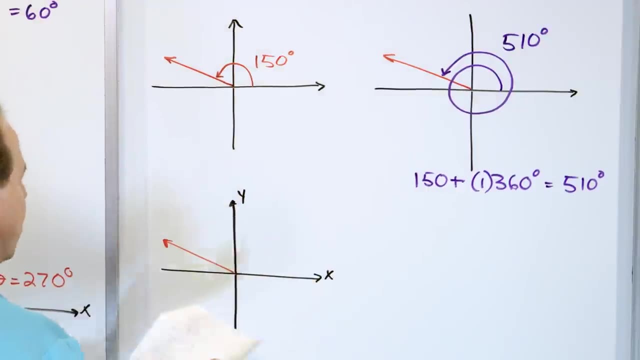 And of course we want to because we're learning right. So we're gonna take and say, well, the terminal side of this guy is the same physical location, but now we're not gonna go around one time, we're gonna go around two times. 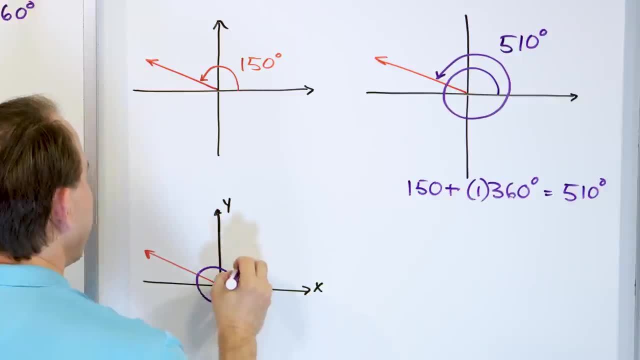 So what we do is we say: well, here's the 150, and then we go around one full circle again, then we go one full circle again back here. So we had 150, then we went another full circle and added 360. 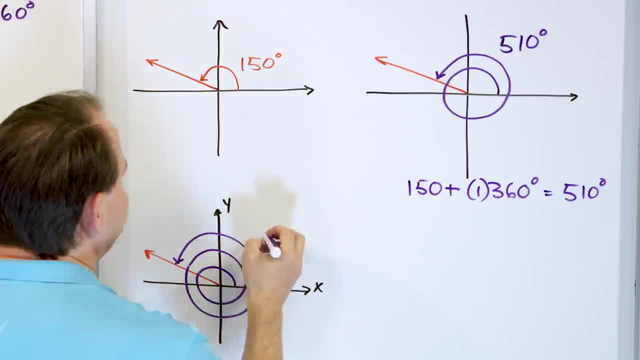 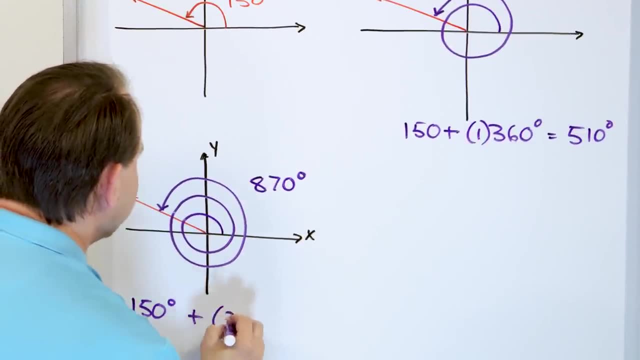 Then we have another full circle and add another 360.. What is that angle measure? That is 870 degrees. How do I know? Because I could take 150 degrees, the initial angle, and I can add to it two circles, which is two times 360.. 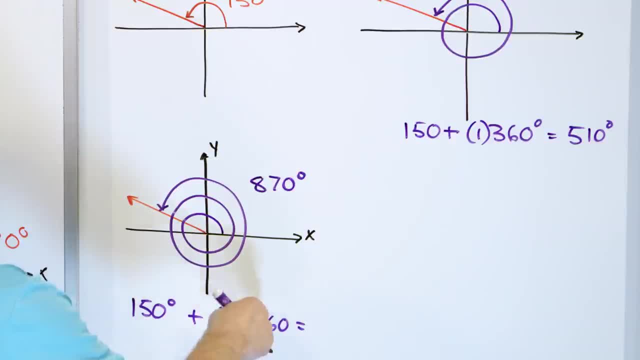 So if you do this on a calculator, 360 times two plus the 150, you're gonna get 870, right? So what we're trying to say is: 870 degrees positive is the same thing as 510 degrees positive, is the same thing as 150 degrees positive. but it's not the same thing. It's this one here. So a 1ad plus a 50 degrees, plus the dodger-huxt one. At this point you the other way around- the other way round- is getting 360.. In this case, instead, 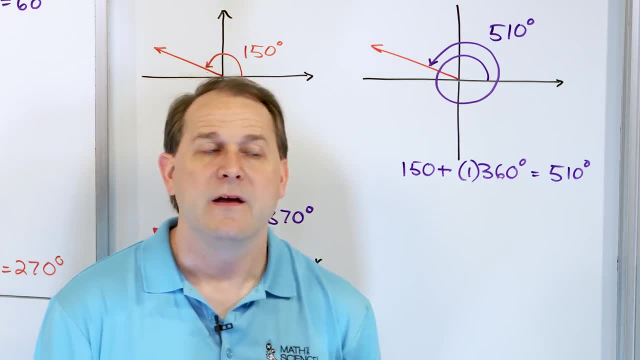 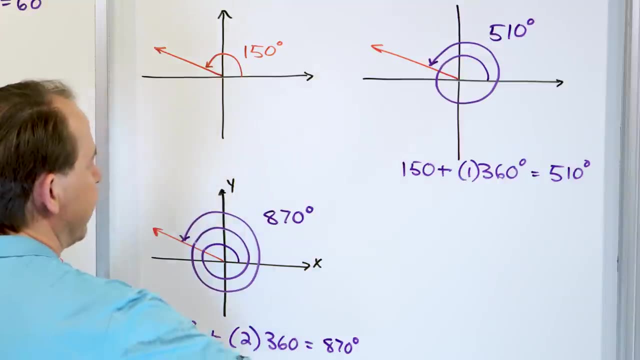 it always expresses exactly the same angle. You're gonna have to get used to adding or subtracting 360 to angles, because you end up having to do it a lot as you study this kind of math. right Now, we've added 360 two times and that was all wonderful. 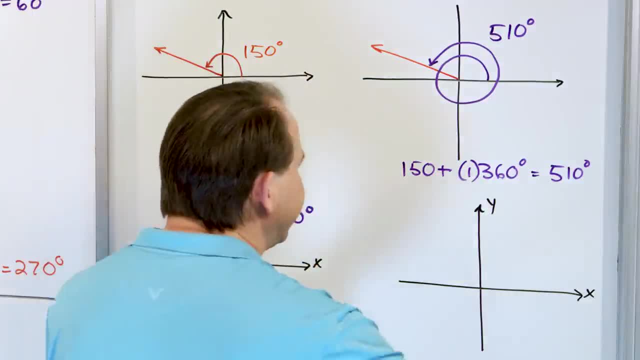 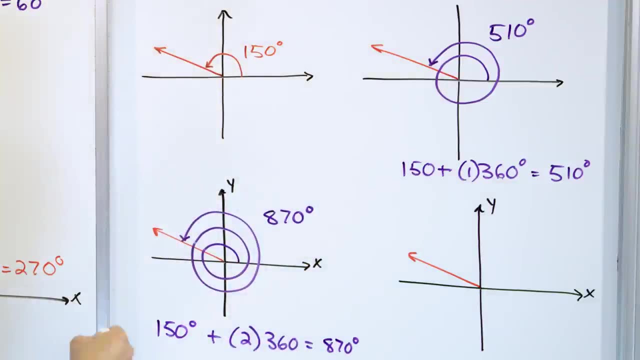 but we can also subtract 360 degrees. There's absolutely no reason why we're not allowed to do that. so we're gonna show an example of that here. Same exact terminal angle as before, but now instead of adding 360, when you add an angle, 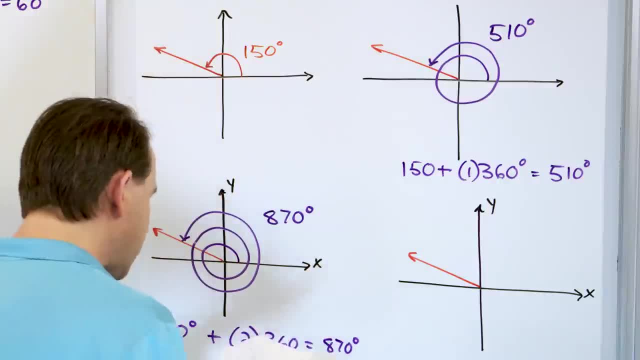 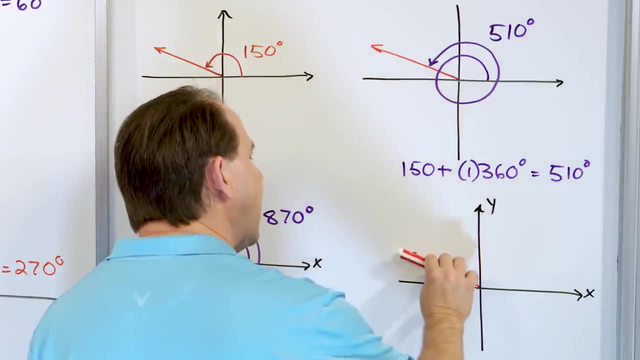 you go in the positive direction of that angle, measure. okay. Here what I'm going to do is I'm going to say: let's, instead of taking a look at this as 150 degrees positive, let's measure the negative angle going down below here. okay, 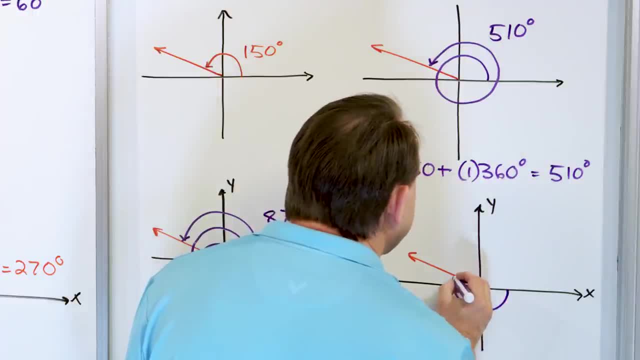 What would that angle measure be? If I start here and I go this direction, how would I get to that angle? What would that angle actually be? Well, I know that this is 150 degrees positive, right, And instead of adding 360, what I'll do is: 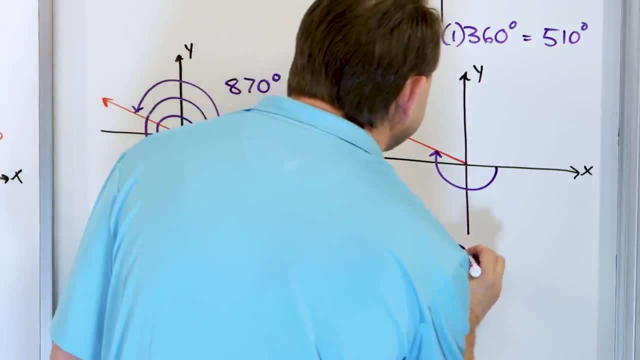 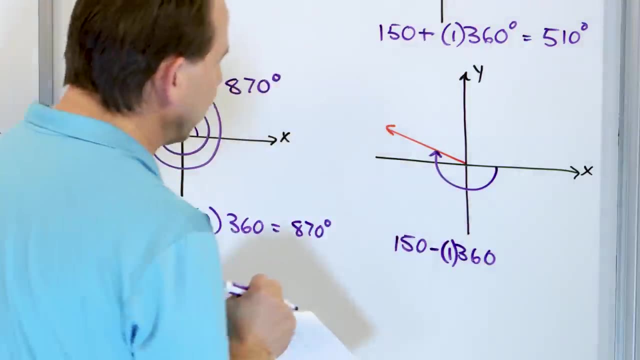 I'll go the other direction and I'll subtract 360.. So I'll subtract 360 degrees from it. In fact, just to make it 100% clear what's going to happen here, I'm going to subtract one full circle one times 360, and when you get that, 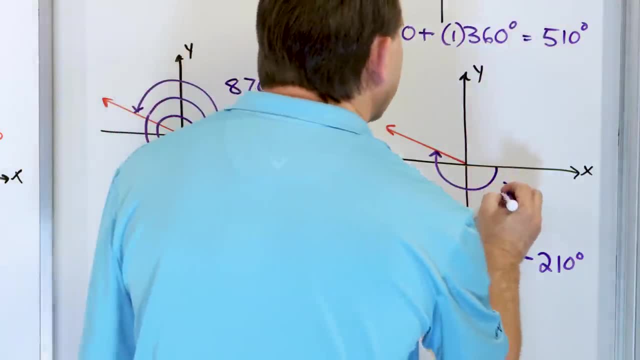 do that and you get negative 210 degrees. So this angle is a negative angle, 210 degrees. It's negative again because it goes down below the x-axis as a measurement. but if you ask me, if I moż, the x-axis is negative or lower. 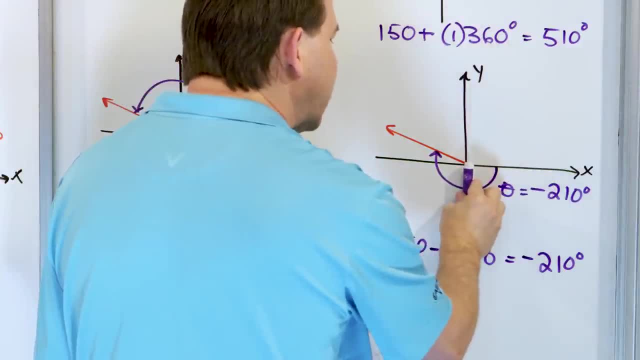 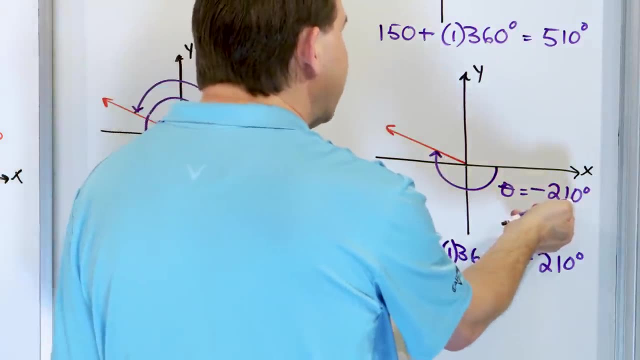 then that would definitely work better. right So" in a clockwise fashion, And it makes sense: This is negative 90.. This is negative 180. And this is just 30 degrees up from that, from negative 180, going in that direction. to give me this, And I 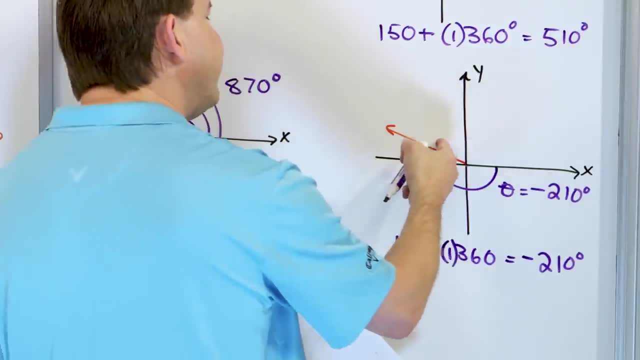 know that this other direction was 150. And so if I add the 150 plus the 210, I'm going to get 360.. So there's many ways of looking at it. Another way of looking at it is, if you know this angle. 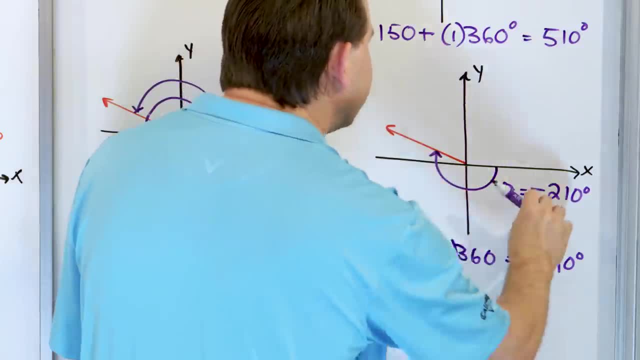 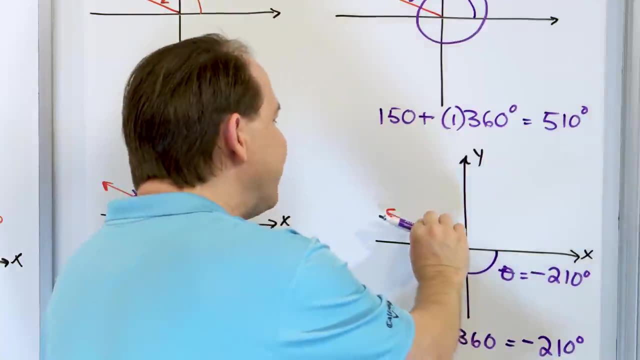 is 150 degrees. like this: instead of adding 360 to get a bigger number, I'll start at 150 and I'll subtract 360. And when I subtract an angle, I'm going to have to go the other way, Remember. 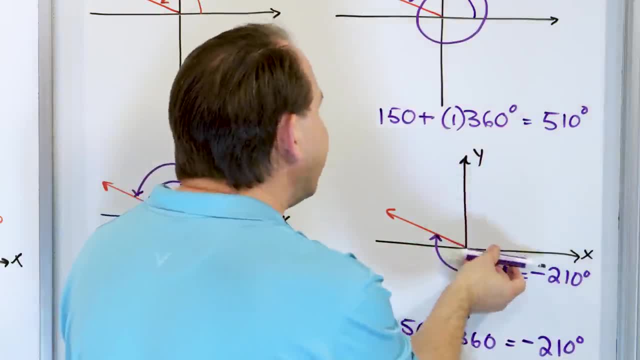 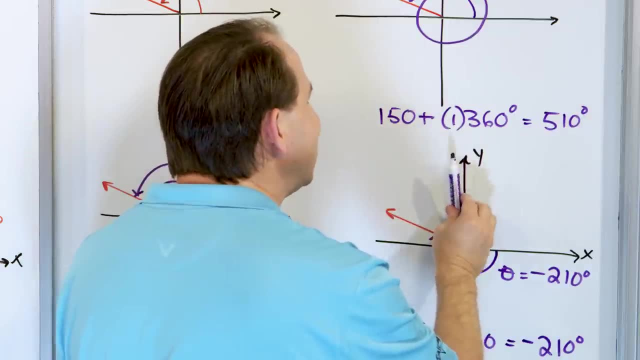 negative angles are measured going clockwise and positive angles are measured counterclockwise. So if I add 360, I'm going to go this way, But if I subtract 360, I'm going to go in the negative direction down here, And so when I subtract 360, that's why the angle turns out to be negative. 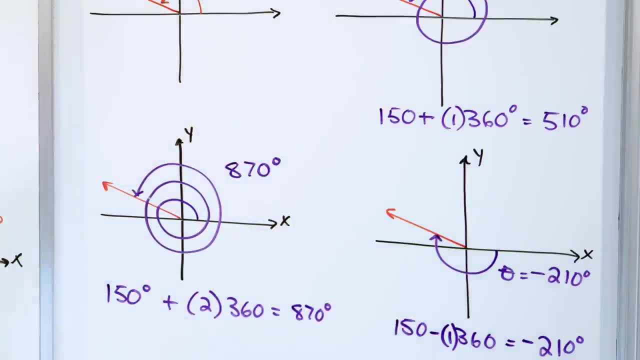 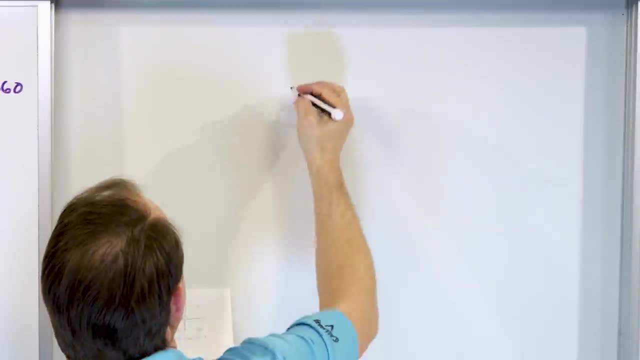 because it's measured below the x-axis, like that. But wait, there's more. I can actually do one more time. I don't need to just subtract. If I subtract 360 one time, I can do it again. Okay, And I'm getting to a punchline. We're almost 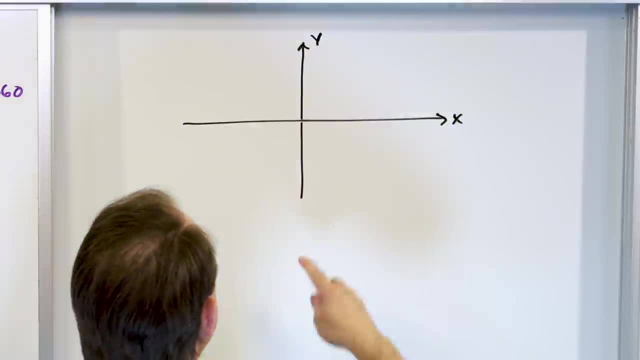 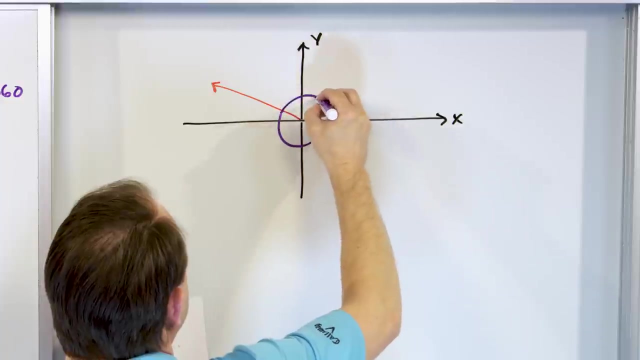 done. But this kind of stuff is really important, this foundational stuff. So here's the terminal side right here. And we went down and we said it was negative 210 degrees. So I can say, well, I can go to negative 210 degrees, but I don't have to stop there, I'll just go another negative 360. 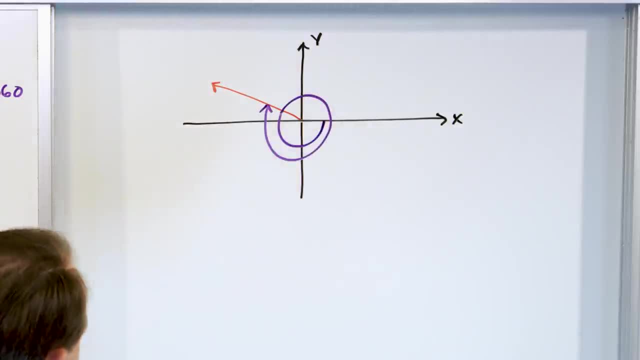 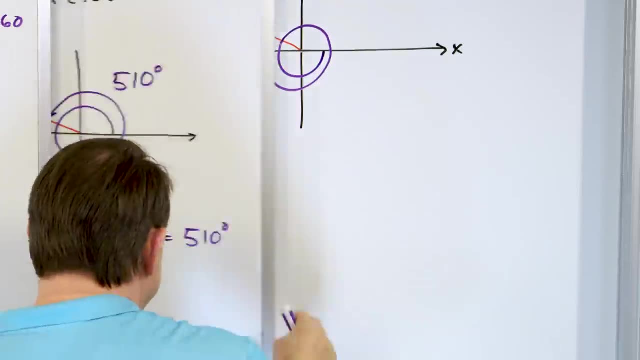 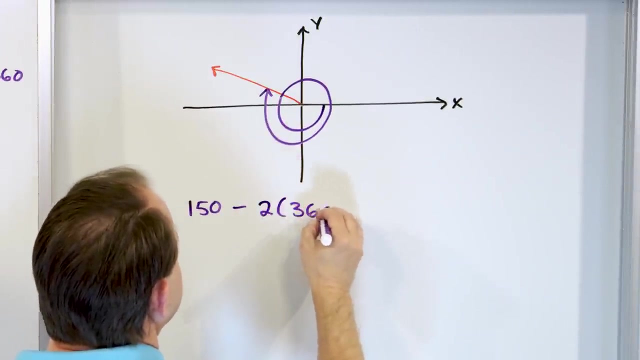 degrees and stop where I be on the terminal angle here. So again I could say: well, I started at 150 degrees positive And instead of subtracting one circle of 360 to get this, I'll just subtract two full circles of 360 degrees. And what am I? 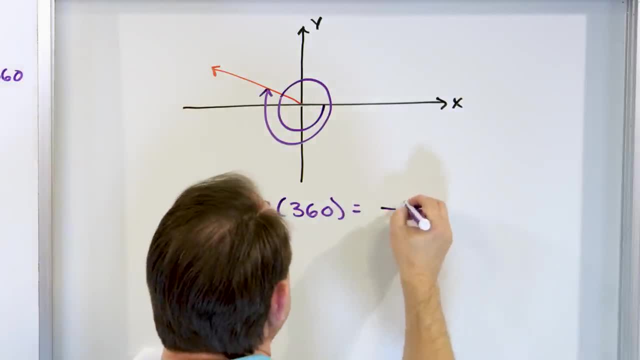 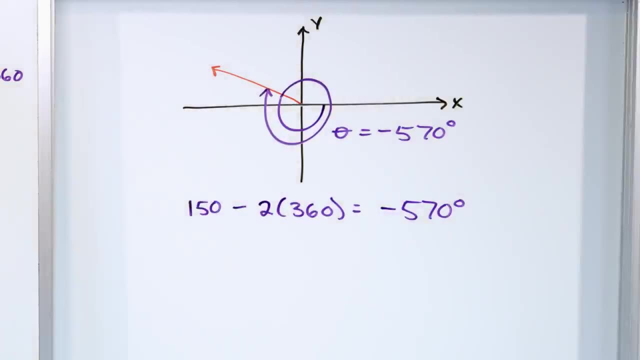 going to get 150 minus two times 360, I'll get negative 570 degrees. So this angle measure is negative 570 degrees. So let's take a minute to really understand what we've done here. What we're basically saying is that 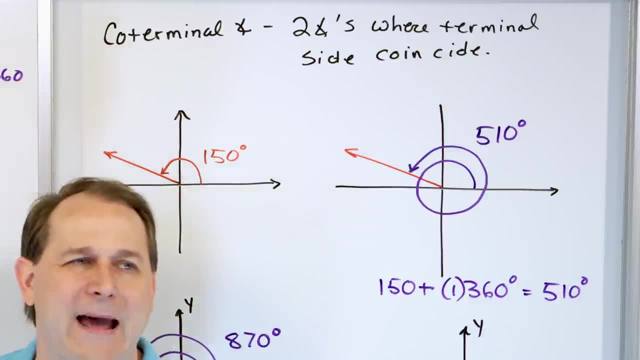 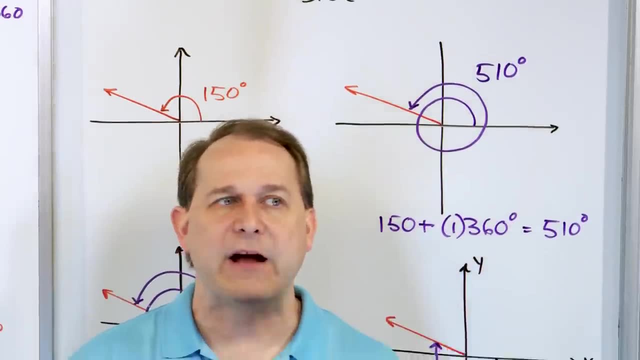 when you look at angles and triangles and back in geometry and more basic math, there are all these little bitty angles that are inside of triangles- acute angles, mostly Okay. But when you get and grow out of that and start talking about trigonometry and pre-calculus, 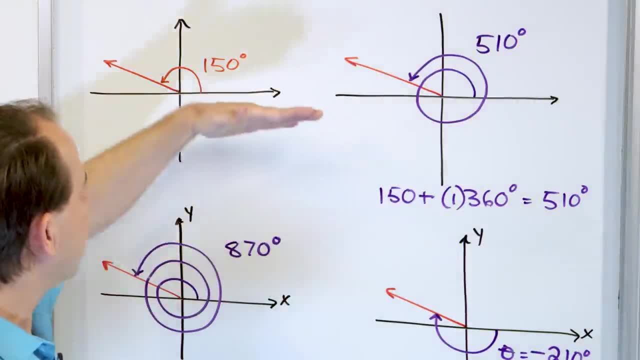 and calculus, the angles become much larger And in general you started an initial position and you define the angle opening positive when you measure this way up to some final terminal position, or you can measure the other direction, going negative angles to the same terminal. 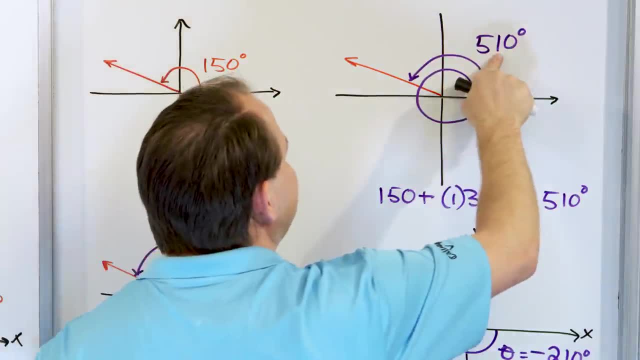 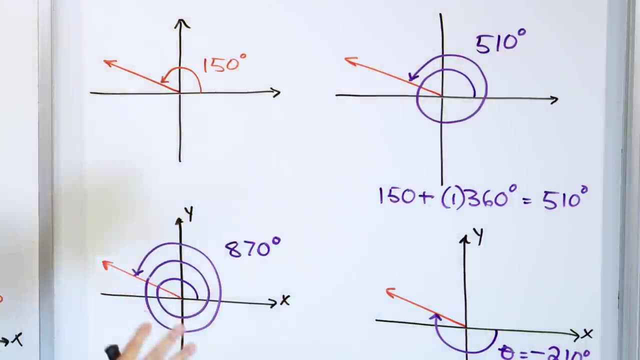 position. Whatever position the angle is in, I can add 360 degrees and get a larger angle. I can add 360 again to get yet another larger angle. but these three numbers represent the same physical location of the terminal side, the angle, which means these are coterminal angles. 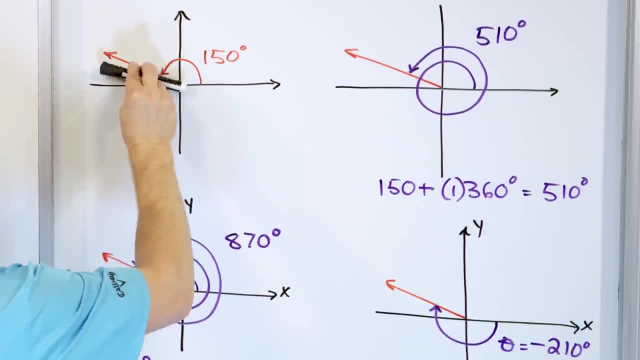 Likewise, I can start at the same location. Instead of adding 360 going this way, I can start this location and I can subtract, which means I go the other way, subtract 360 going here, And when I do that subtraction, I get a negative angle which also again represents the same. 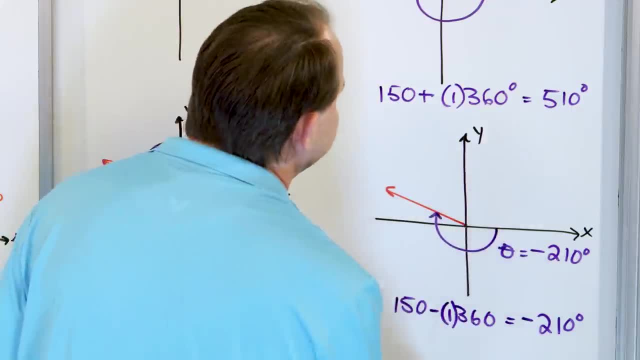 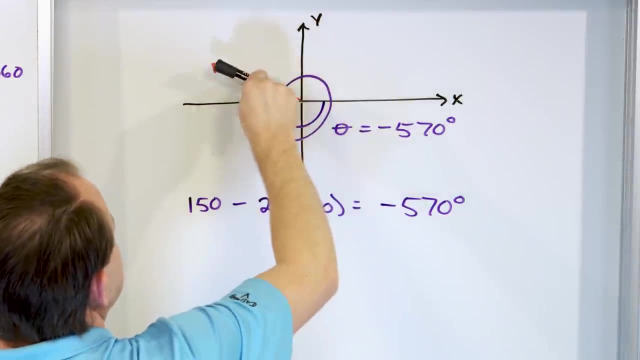 physical thing. But I don't have to stop There. I can subtract another 360 if I want to. So I can start here and I can say, well, okay, I'm going to subtract 360.. And then I'm going to subtract 360 again, from this angle again. 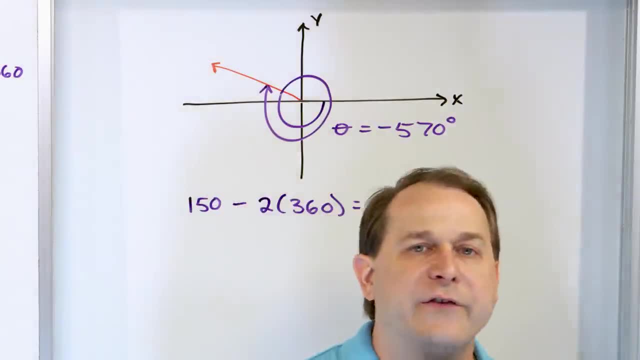 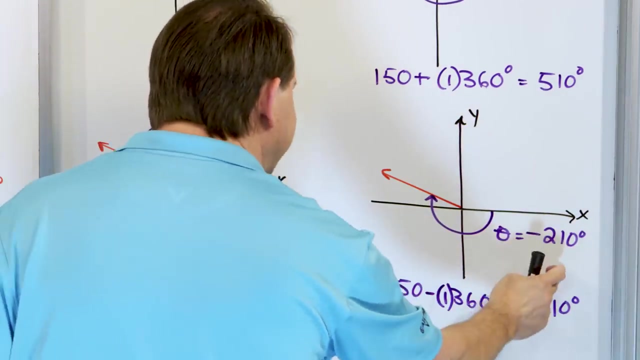 subtracting two full circles, I get negative 570.. So I can add as many 360 degree cycles as I want and get the same coterminal angle. or I can subtract as many 360 degree cycles as I want and get exactly the same coterminal angle. This angle is exactly the same thing as this angle. 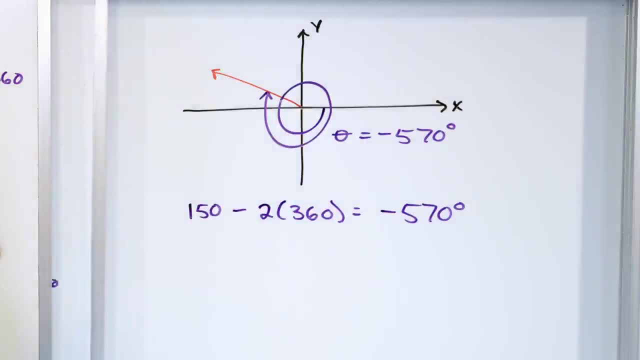 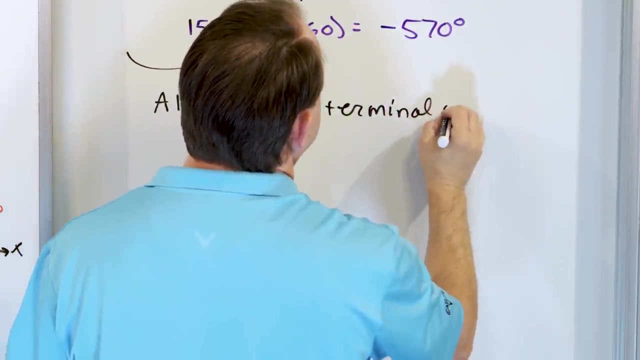 is the same as this, this, this, They're all the same. Okay, They're all the same. That's all I'm trying to say. So, to summarize the whole thing, what we can really say is that all angles, coterminal with 150 degrees, can be written as follows: 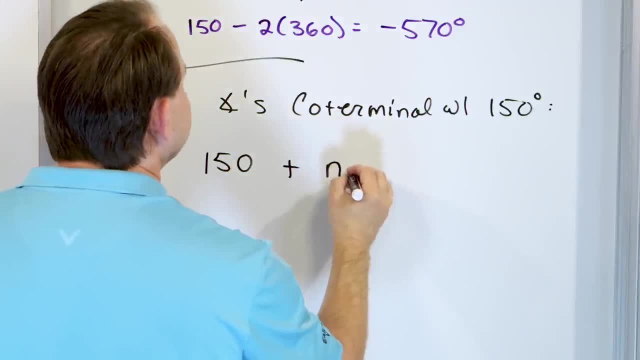 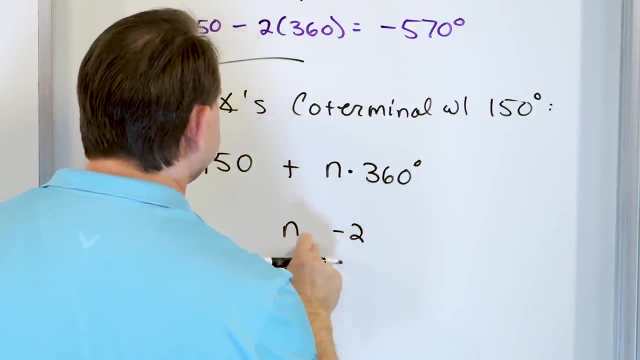 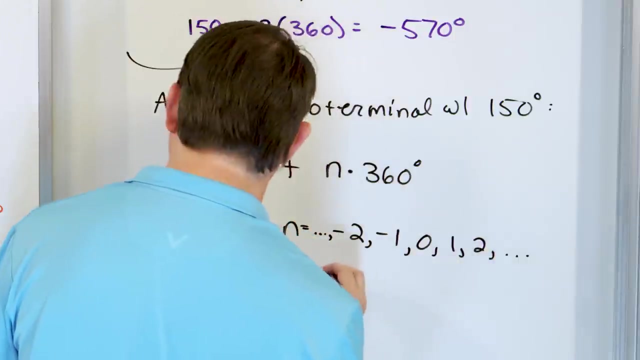 150 plus n times 360 degrees, where n can be negative two, Let me do it this way: dot dot dot, negative two. negative one, zero one, two dot dot dot. So what it means is all. 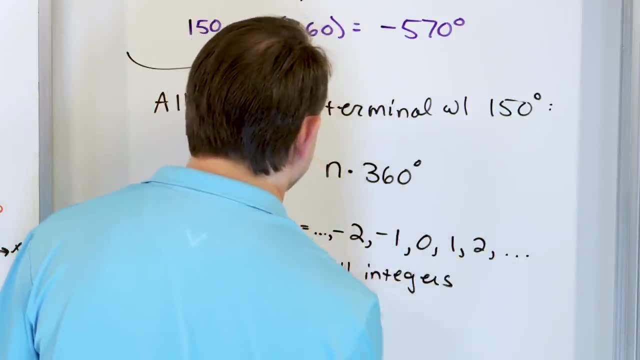 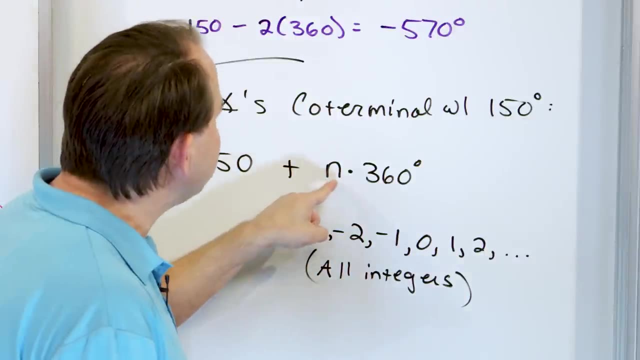 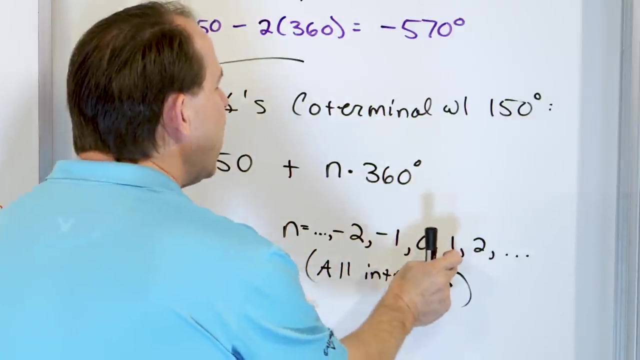 integers. In mathematical terms, what it's saying is: you start with some kind of baseline angle and I can add as many 360 degrees to it as I want. If I add zero 360s to it, then I just have my original angle. If I add one 360 to it, then we did those on the board. If I add two and three, 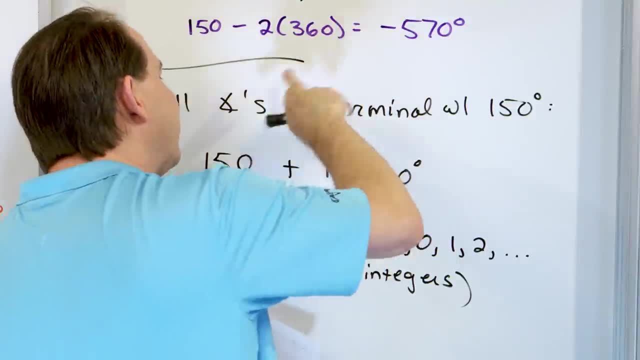 and four and five. we're going to get the same angle, So I can add as many 360 degrees to it as I want. I can get bigger and bigger numbers, Or I could subtract 360 going the other way. negative one, negative two, negative three and so on. So there's an infinite number of ways I can.